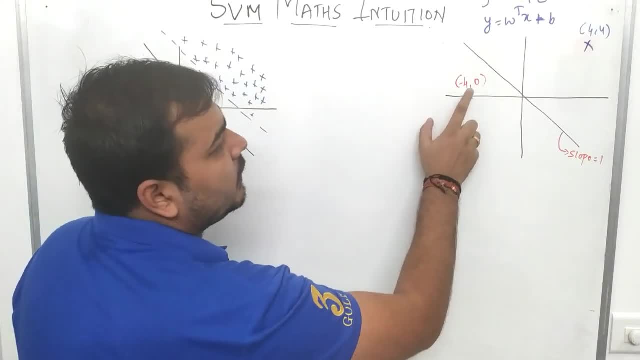 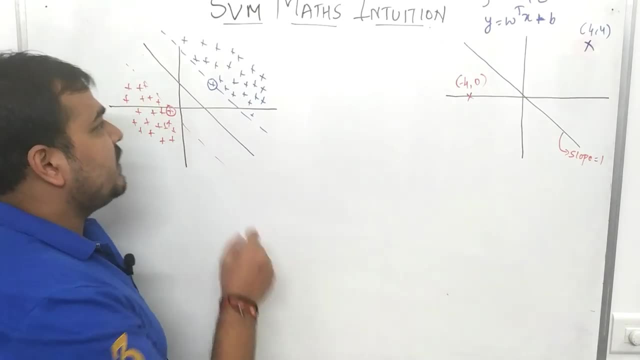 example, guys over here. Okay, I have two points. that is minus 4 comma 0 at this particular coordinate and there is 4 comma 4 at this particular coordinate. And suppose I draw a particular point In this particular case. I'm going to say that suppose consider that. 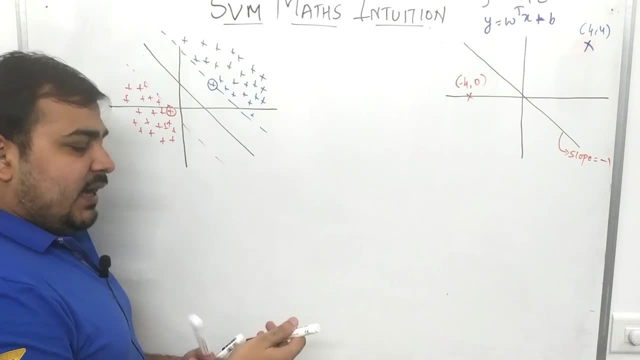 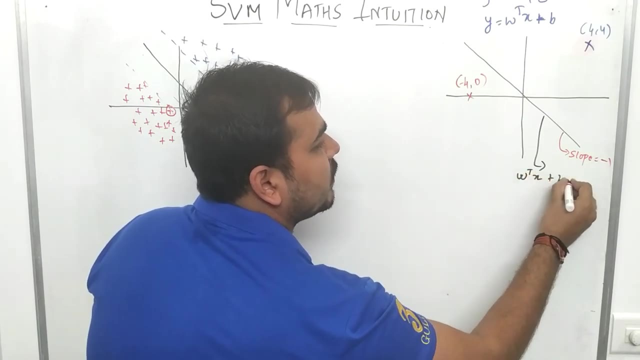 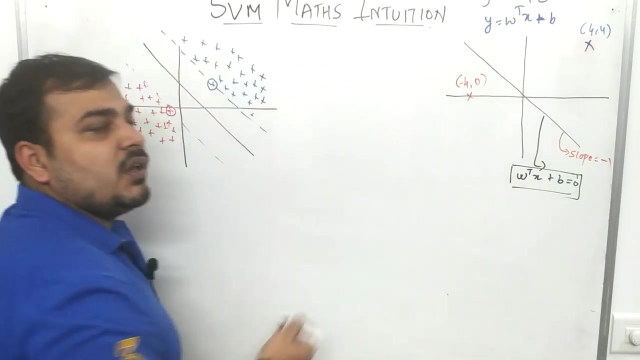 my slope is minus 1.. Okay, And you know that the equation of a hyperplane, of this particular hyperplane it is given as w transpose x plus b, is equal to 0.. I hope everybody is familiar with this because I have already discussed this in my logistic regression. If you go, 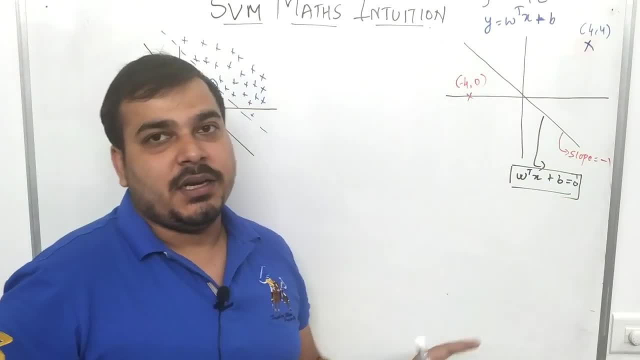 and search for what is the equation of a hyperplane. we basically get this particular equation right And we also know this particular equation right. y is equal to mx plus 5.. So we basically get this particular equation right And we also know this particular equation right. 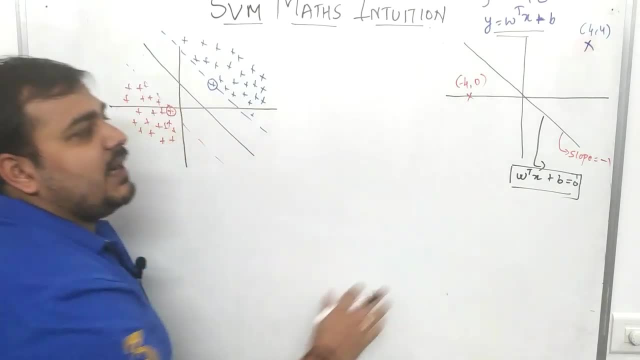 x plus 5, right, Everybody knows that. Now understand this thing, guys. Suppose: for this particular coordinate, I want to calculate the y value. How do we calculate In this particular case? I know my slope, that is, my m, is nothing but minus 1, because I've just 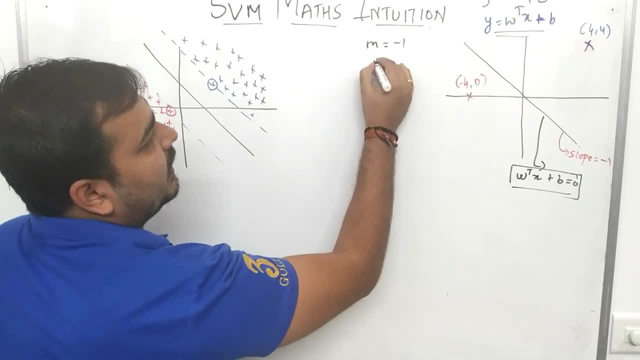 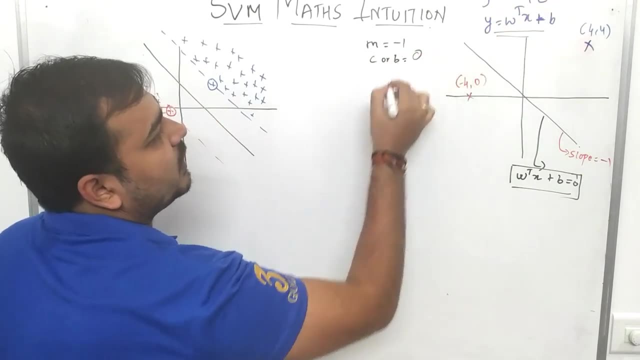 considered this as minus 1.. You can see right. The next thing that I have to do is that what is my c value or b value? Okay, So this c or b constant, this is going to become 0 because it's passes through the central origin coordinate. 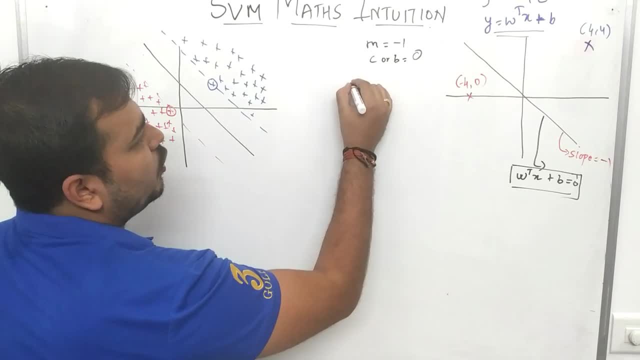 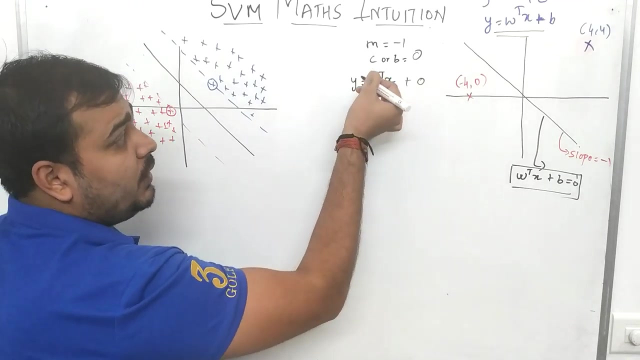 Right, It passes through 0. So I'm going to consider this. So, in short, my equation becomes: w transpose x. Right Now, with respect to this w, okay, and this c is basically zero, If I want to do this particular multiplication, and I have to do the W transpose multiplication. 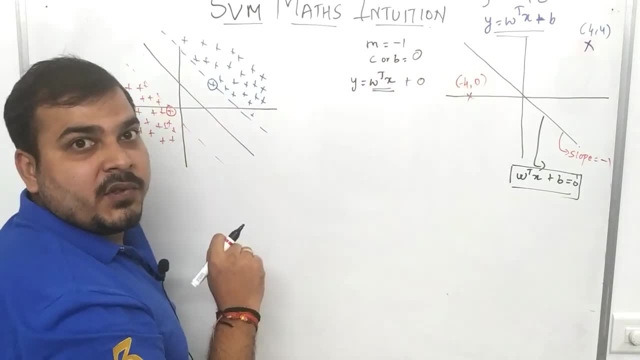 of x, x. I have two coordinates for this particular point, Right, So I have: this is my x 1, this is my x 2.. So consider this as my x 1 and this as my x 2.. Right, of course, this will. 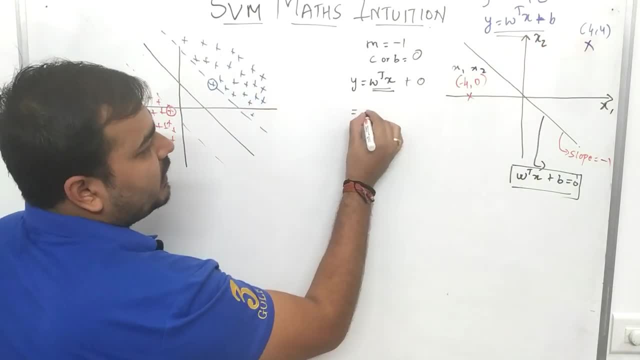 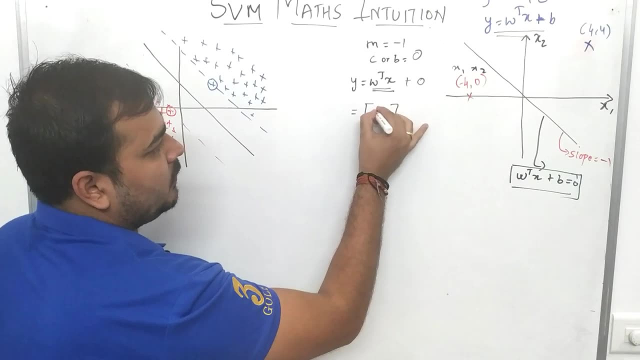 change for you guys as well. Okay, right. So if I want to make this multiplication, what is W over here? in this case, W is nothing but slope right. Slope over here is minus 1, right, And if I consider this B as 0,, this: 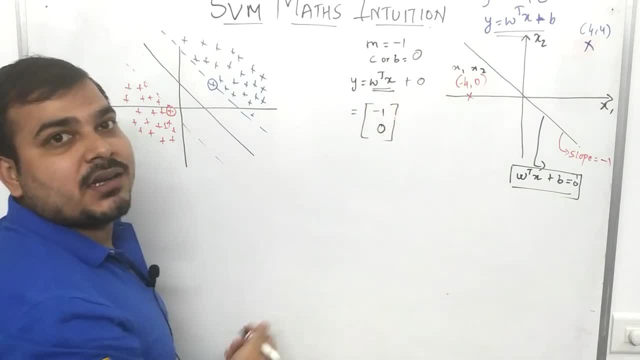 will be my 0 over here And why I am doing transpose? Because I have to do the matrix multiplication. And suppose, if I take my x coordinates, that is, x1 and x2, this is nothing but minus 4 comma 0, right 4 comma 0.. Now if I want to do the matrix multiplication, 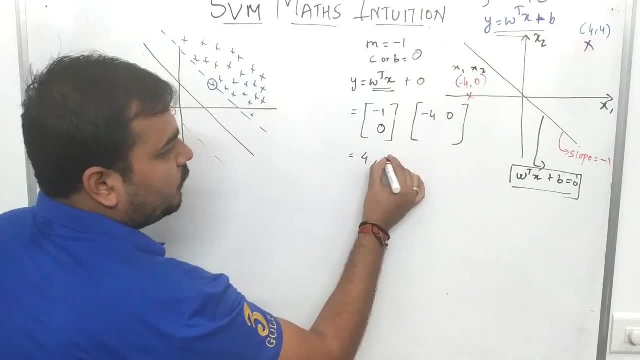 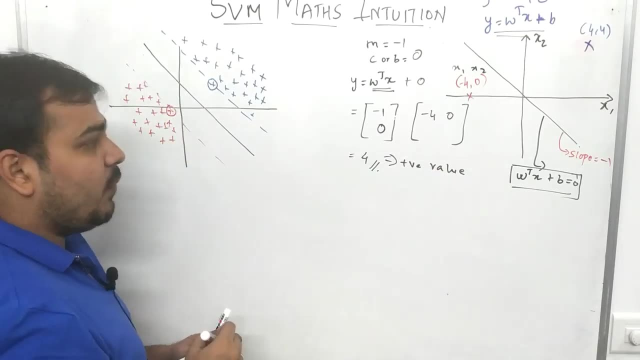 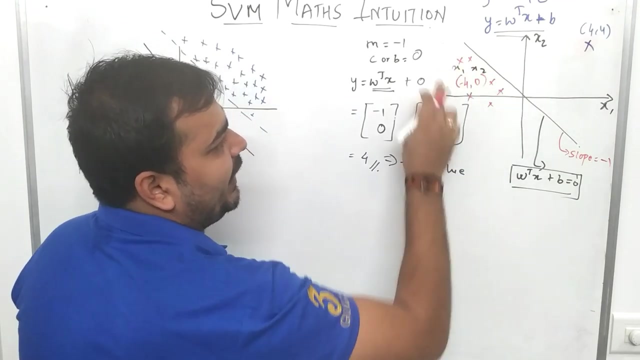 you will be seeing that my value is 4, right, This 4 is nothing but a positive value. Now, with respect to this guys, understand one very important thing. Let me come up with any other points over here, any other points over here before this particular line, and 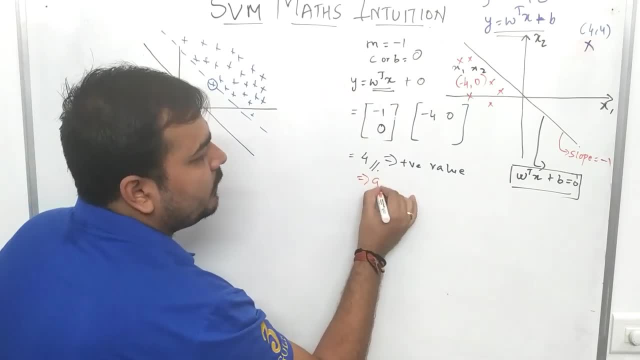 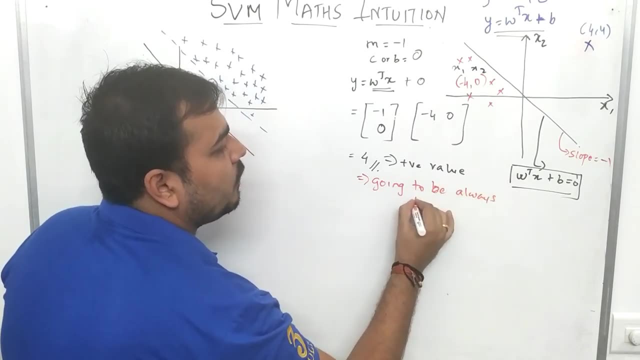 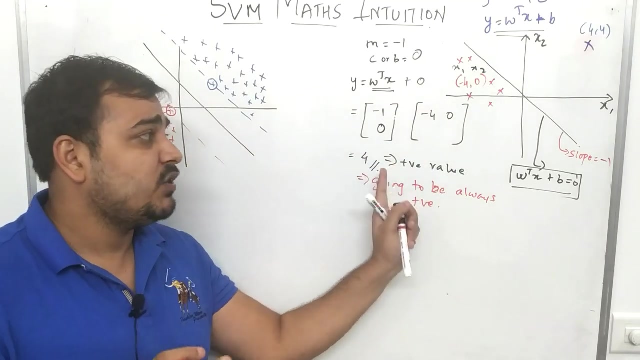 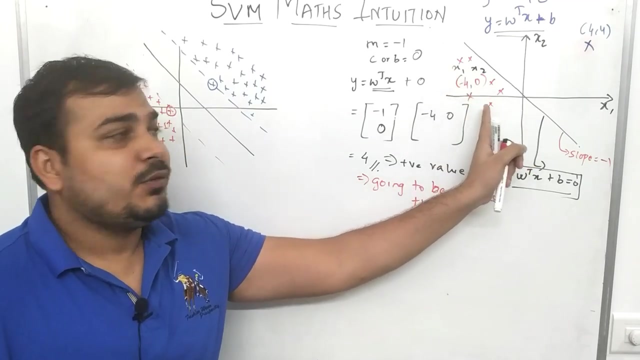 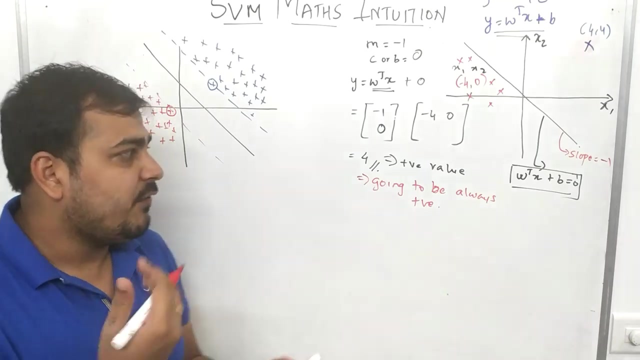 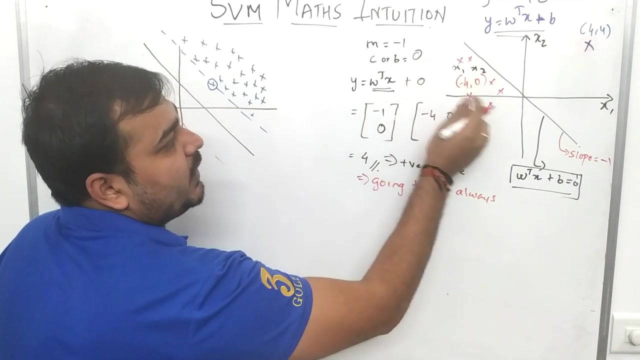 if I try to compute my y value, it is going to be always positive. It is going to be always positive, Okay, Okay, Okay. and this particular thing, when I was explaining logistic regression also, I missed this thing, So I'm trying to explain you over here. Whenever we go below this particular line, in this situation over here, with respect to this particular points, whenever I'm trying to compute in this particular equation, at that time you'll be seeing, my y value is always going to be positive. Okay, it may differ, It may become 4,, it may become 8, it may become 9.. But what is the main aim? Anytime I come up with respect to this particular points, it is going to be positive, Okay, so this is. 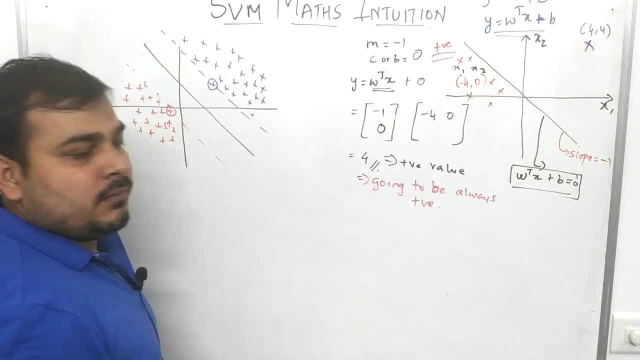 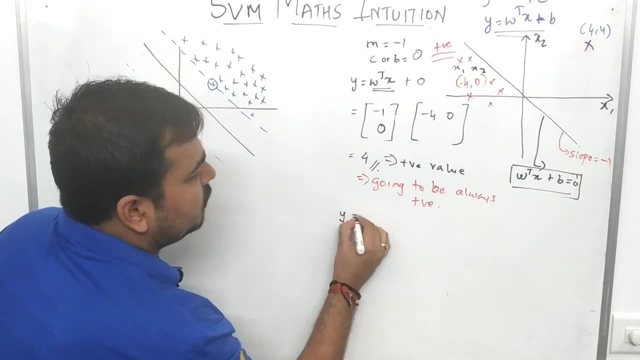 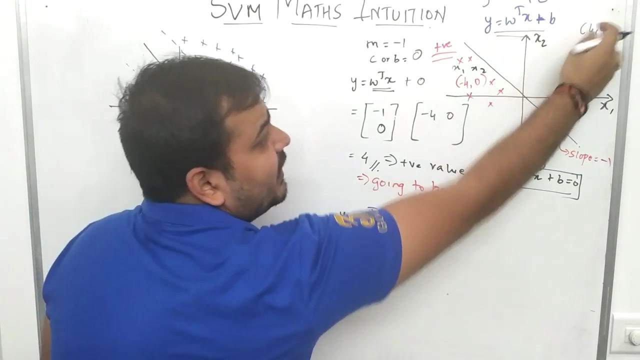 one scenario. Now suppose for this coordinate, if I calculate- Okay, suppose I go above this particular point and I do the same computation. Right, y is equal to w. transpose x. Now, what is my w? It is same minus 1, 0.. What is my x? x1 and x2.. It is nothing but 4, 4.. Now, 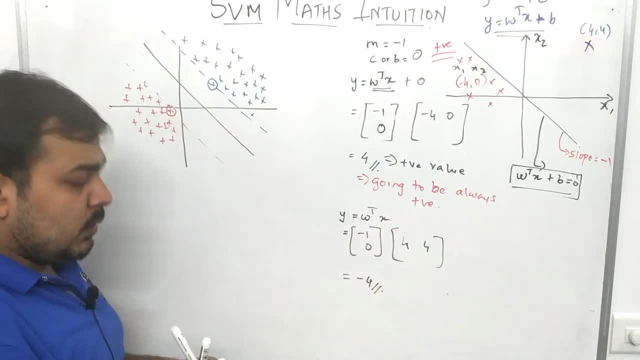 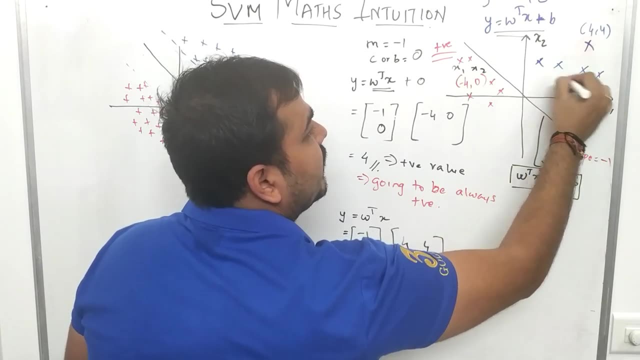 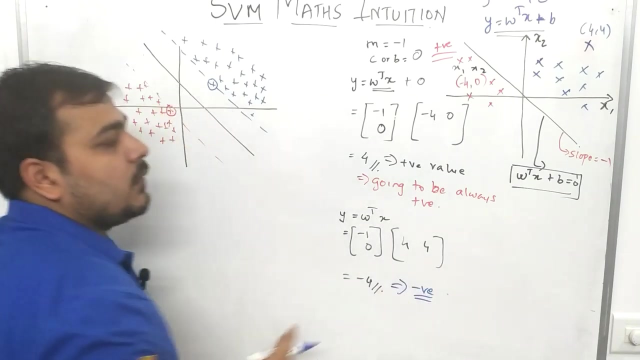 if I do the calculation, this is going to become minus 4.. Now, if I come up with any points at that side, If I try to come up with an equation over here, or if I try to find out the y value, it is always going to be negative. Okay, so this basically indicates that on this line, when 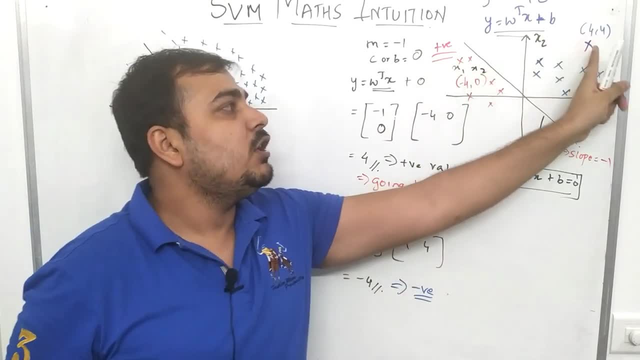 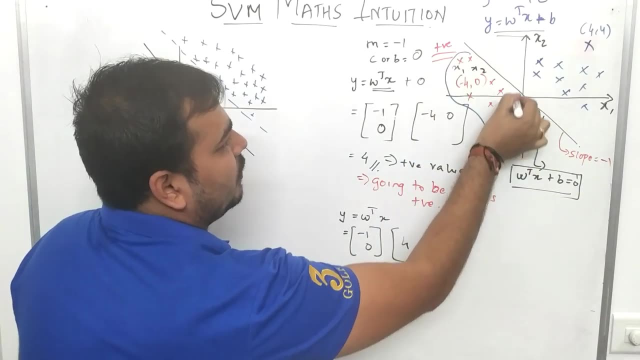 I'm coming towards the downward direction, these values are positive. When I go on the topward direction, we are getting a negative values. So here what I can do is that I can consider this as one group, this as my another group. Okay, but still, the question raises: 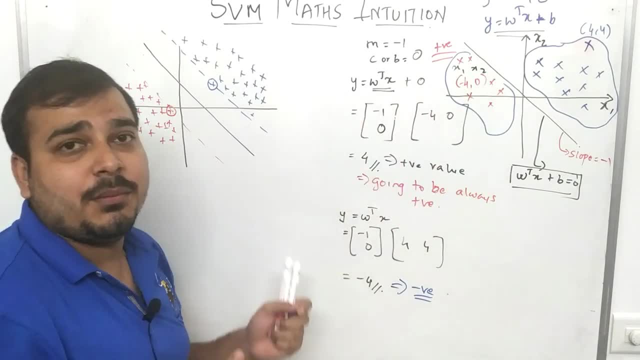 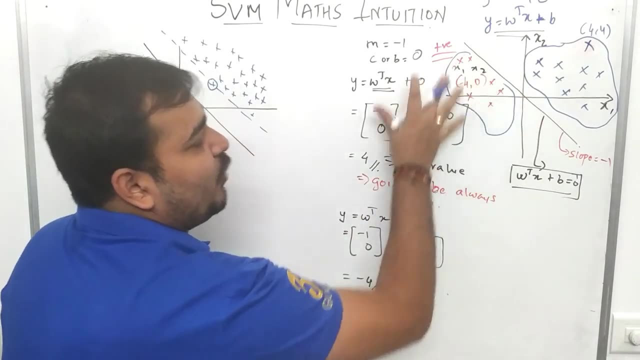 is that We are getting positive and negative value, Why we are discussing about this? Right, because it is important. In SVM, we will try to understand why it is important. Okay, so this is one group. this is my another group. When I say positive, can I consider it as plus 1? See. 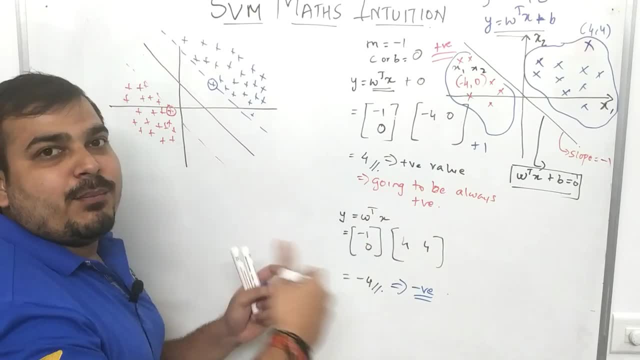 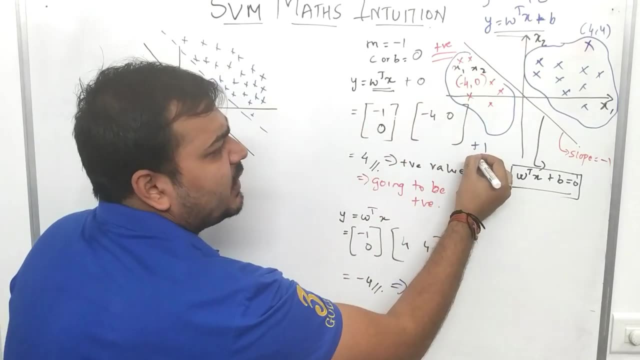 anyhow, it is going to be positive. Okay, it may be plus 5 plus 6, plus 7, plus 8 plus 100, but it is positive, Right, and since, in a classification problem, I can consider this as plus 1. Because it is a positive value. Okay, just to simplify my 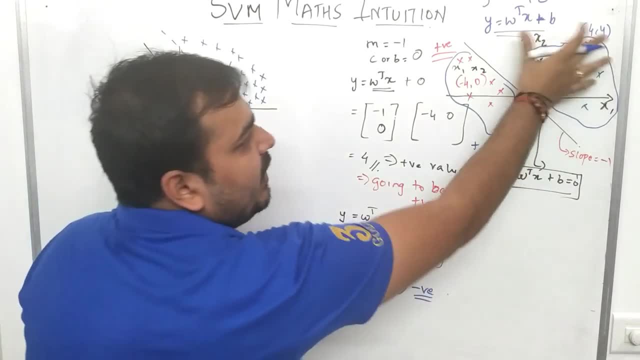 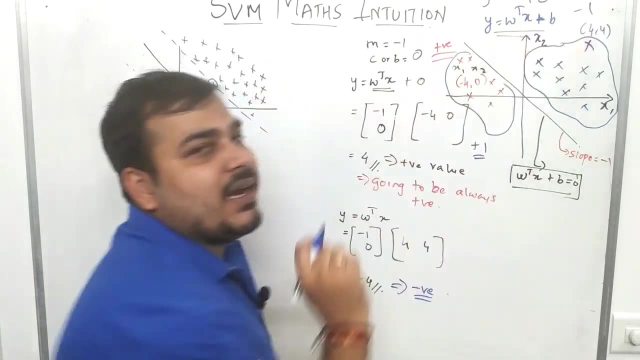 derivation and forward how I am actually going to treat it. And similarly over here, since this is negative, I am going to take it as minus 1.. So this whole classified point is plus 1,. this whole classified point is minus 1.. That. 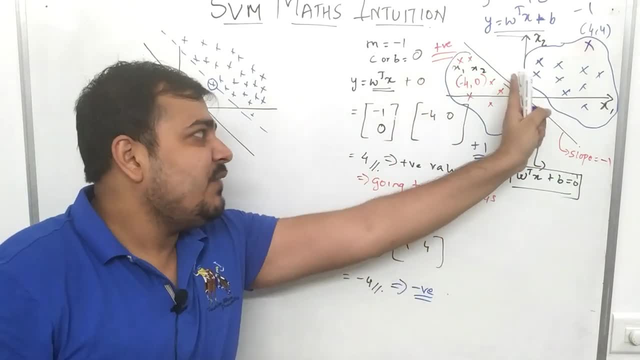 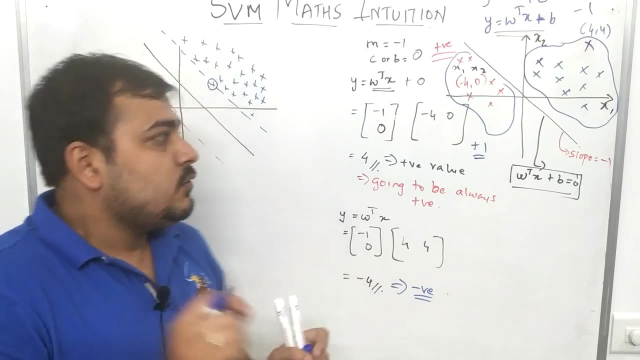 is simple, pretty much simple, Right, and this particular line basically says that if I go below this, it is going to become plus 1.. This is one of the category: If I go above this, it is going to be minus 1.. Right, so, understanding this particular situation. Now, over here, my 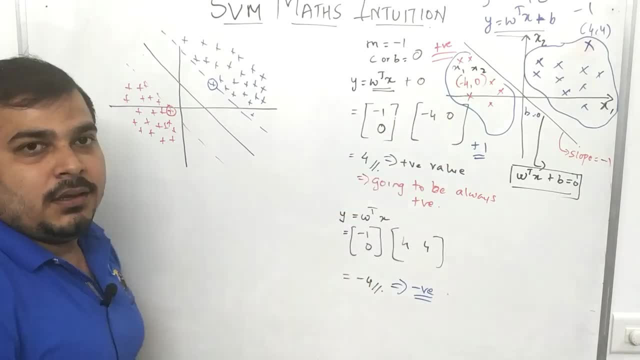 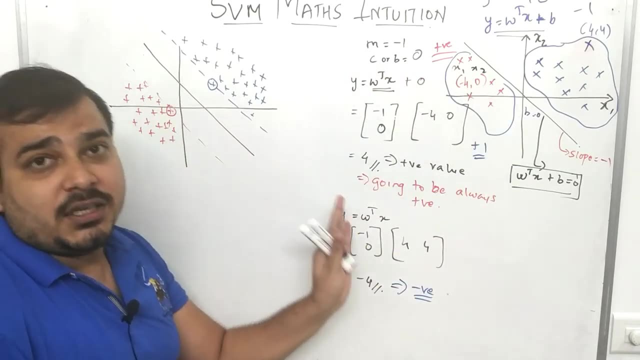 B is actually zero. Right, this B is actually zero. My, this particular intercept is actually: Okay, now, pretty much simple. I have done this. You have understood why we are taking this as plus 1 and this as minus 1. that you have understood. 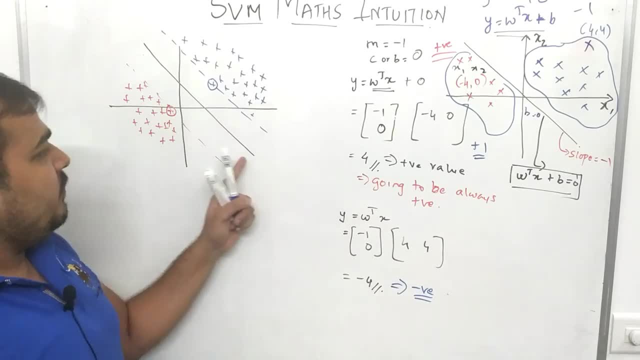 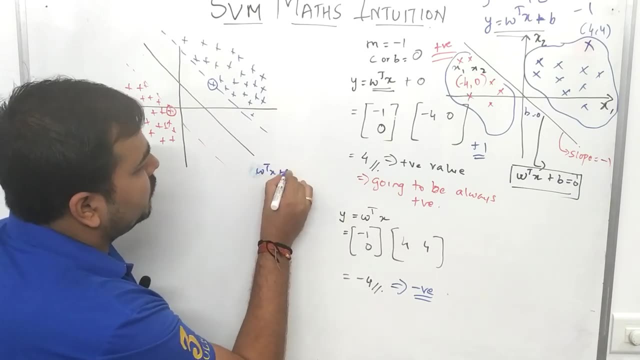 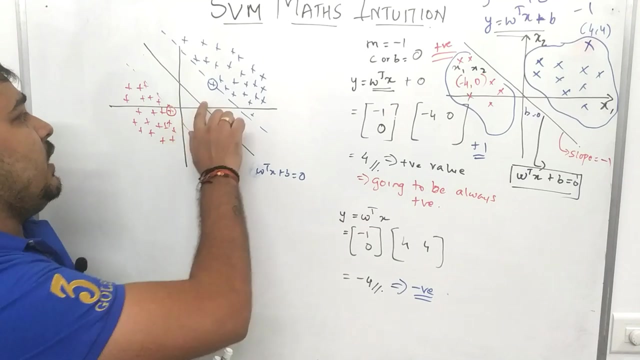 Now let us go ahead towards SVM. in SVM, This particular equation. as I told you, this equation can be given as: W: transpose X plus B is equal to 0.. Okay, So this is one of my equation that I have written over here. Now what I do is that, from this particular point, 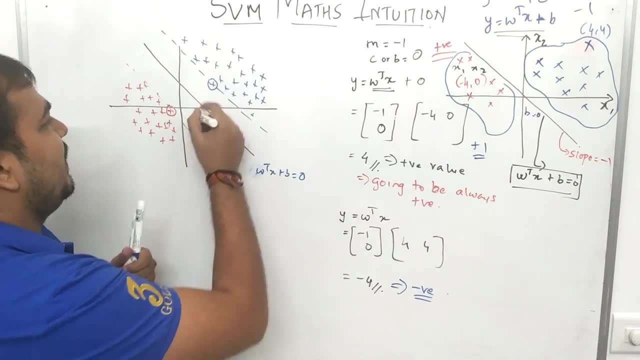 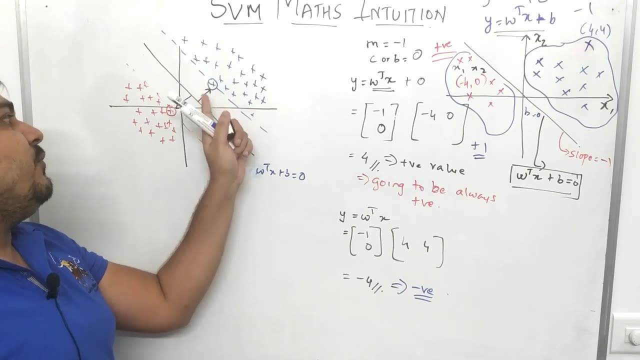 I'm just going to stretch my hands, suppose, from this point I'm just going to stretch over here and from this point I'm just going to stretch over here. So I am going to find out the nearest point over here. Okay, nearest point is basically this blue point. right, As soon as I find out this nearest point, I'm just going to draw the. 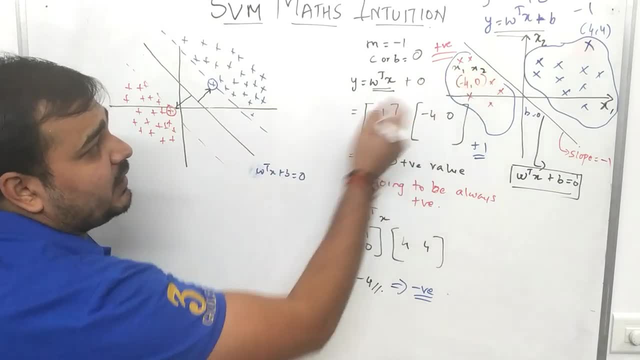 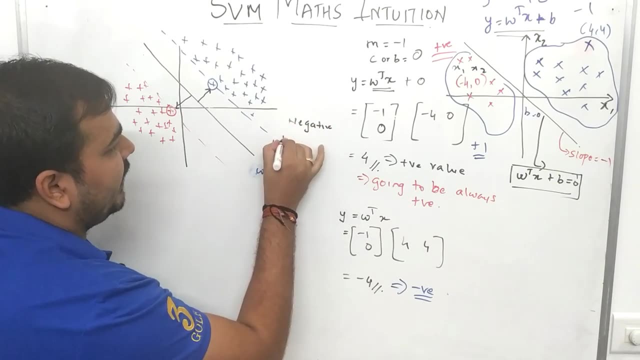 marginal plane, so this will become my. In this particular scenario, this will become my negative plane. right negative plane, Now negative plane. I can basically write this Equation as W transpose: X plus B is equal to minus 1. Okay, so this is my another equation and, similarly, in this particular scenario, I can basically write it as: 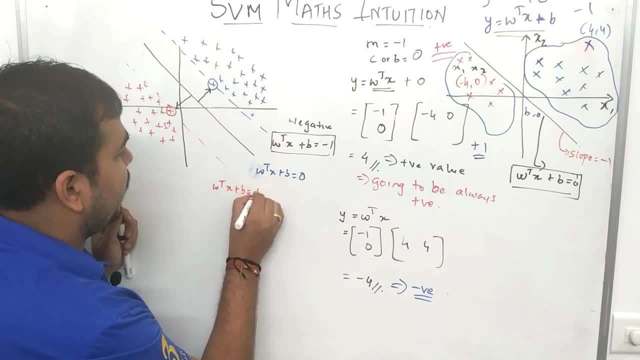 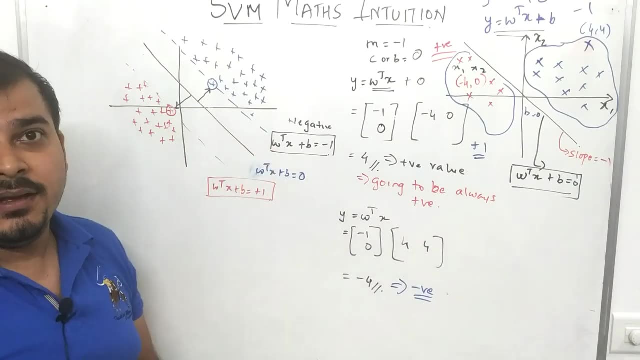 W. transpose X plus B is equal to positive 1. So let me consider two planes, and this is my marginal plane right in SVM We have to compute this marginal plane right and based which will like, based on a problem scenario, Which will be having the maximum distance between these two. 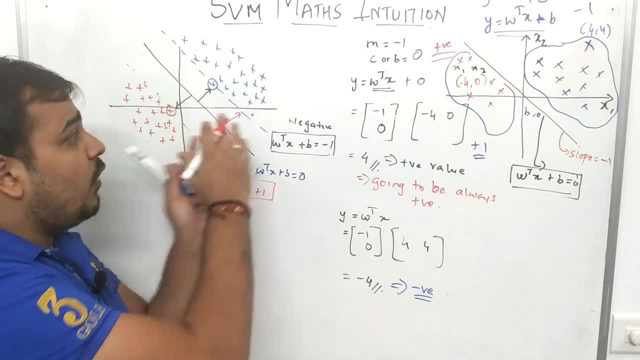 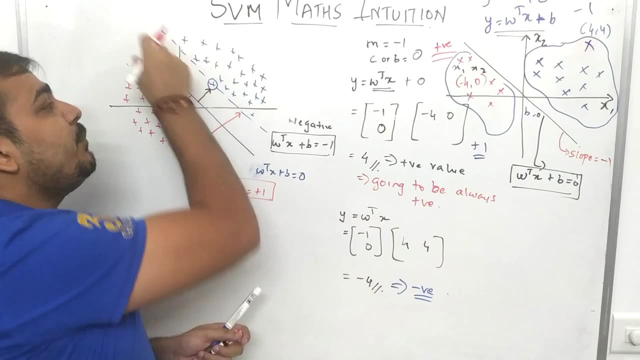 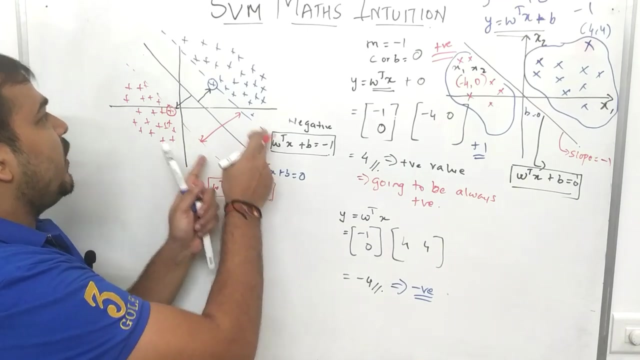 Will be considered the you know best line for dividing this particular points. right, We because understand, guys, this central line is only not. we are not just not actually computing this hyper plane, We are also computing this positive and the negative plane right in SVM. Otherwise, just imagine if you're not computing this. this is just like a logistic regression. 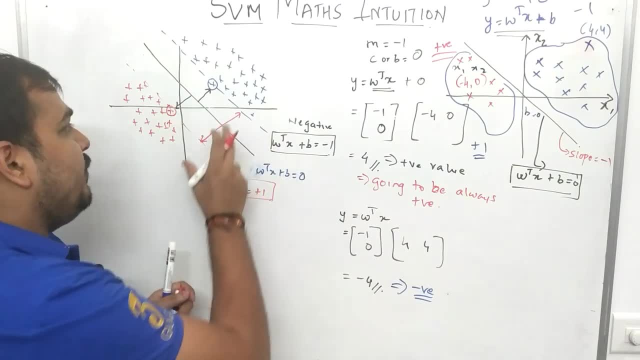 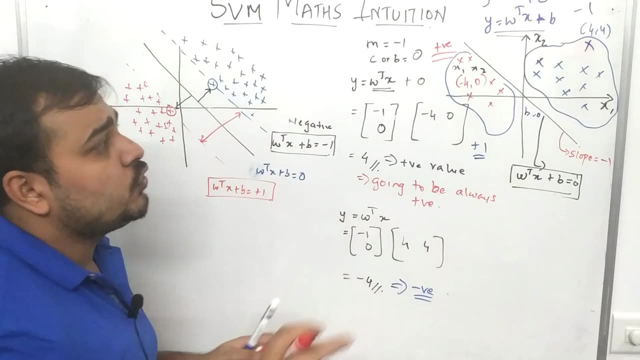 These two things are there, So we need to compute this and we need to have the maximum distance point right. Pretty much simple. Now I have got this particular equation And I have also shown you how this equation is actually valid with respect to minus 1 and plus 1 again. 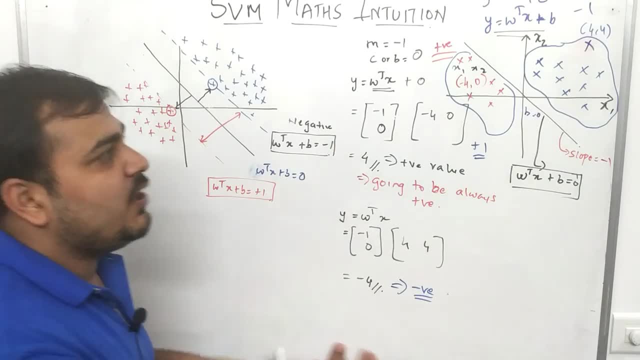 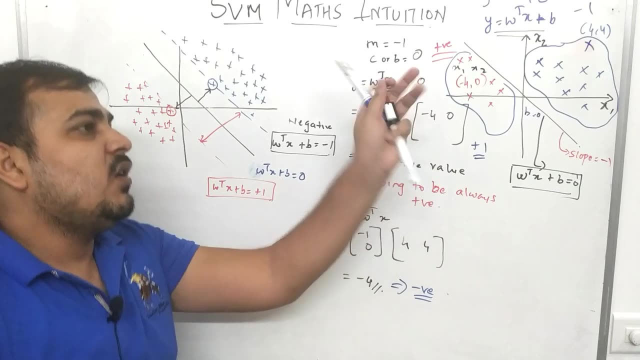 I can have minus 100 or plus 100, but that is not the main scenario over here. I'm just want to find the positive in the negative points. right, We don't understand in real world scenario if I say yes or no. I cannot say that okay, below this line. 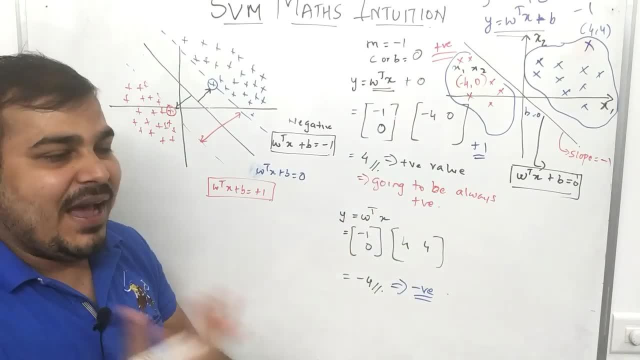 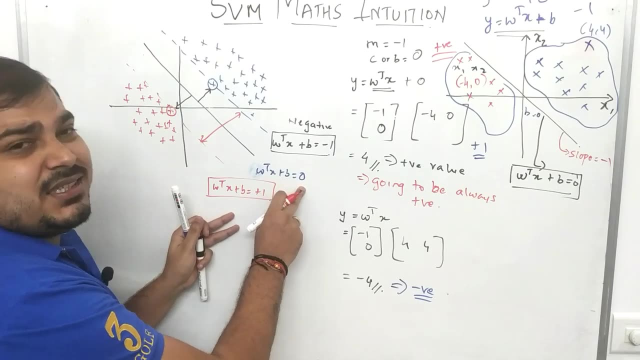 It is yes after that particular line. It is no, Mathematically how we will say, it will actually consider in this particular scenario. So three things. I have told you how we came to this particular equation. This is basically the equation of a hyper plane. 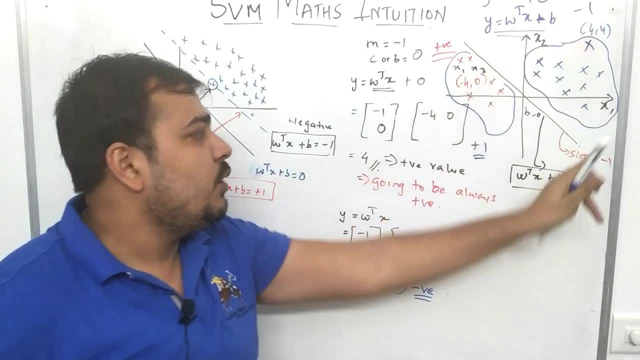 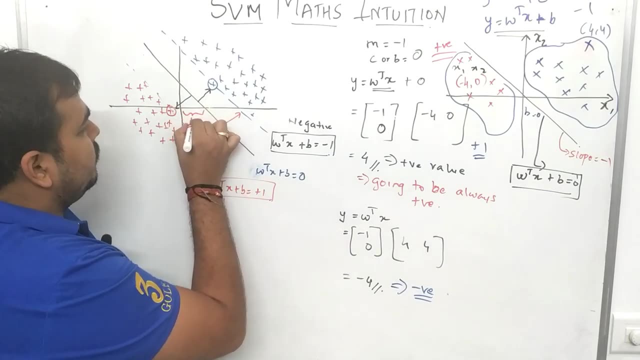 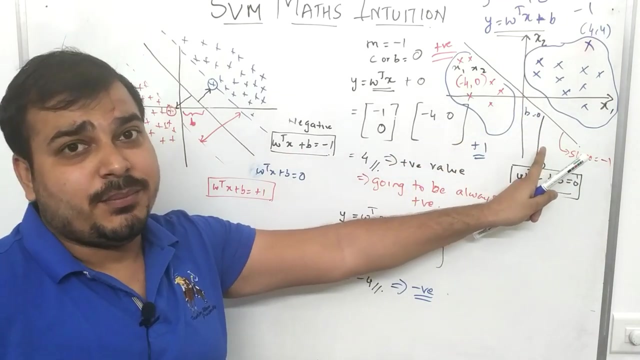 this is Equation because, above this particular points, I have shown you whenever I am computing with respect to the Y value, with respect to anything. and remember, over here I have some B value. The B value is not 0 because it is not passing through the intercept. Okay, there will be some B value over here. B was passing through the 0 intercept, right? 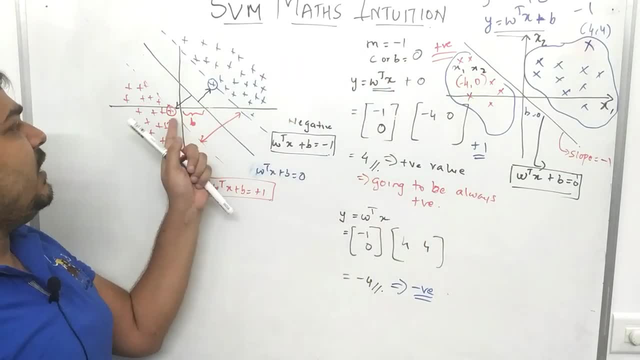 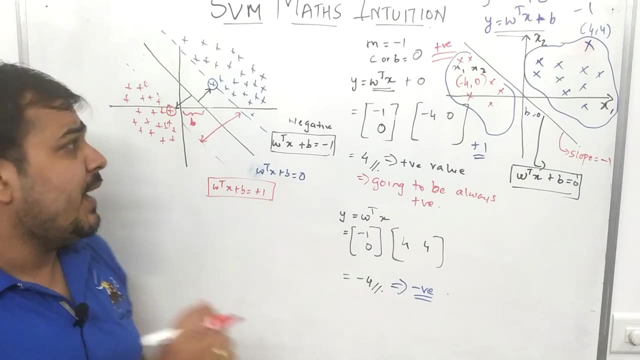 I mean 0 point. so over there the B value was 0, but here there are some distance. Okay, perfect, now we have understood this, But still I told you that in SVM, wherever this marginal distance will be High, that particular hyper plane I will be considering. So how do I compute this right? How do I compute this? very simple. 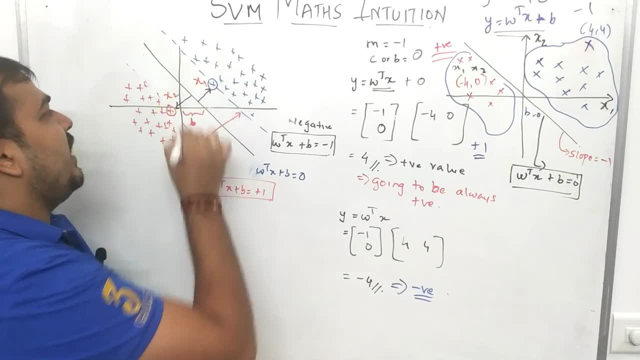 Let me consider: this is my X 1. This is my X 2.. Let me just write in black markers so that you will be able to understand it clearly. Okay, So what I am going to do? Let us consider: this is my X 1.. This is my X 2. 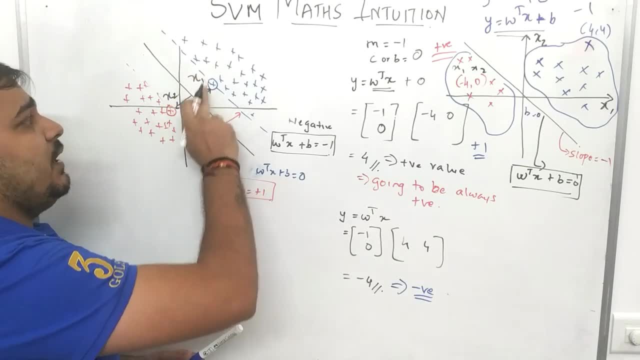 Okay, I want to compute the distance between this particular point and this particular point. if I, if I I mean when I am saying That by this particular point I basically mean this hyper plane and this particular point, I basically have to compute this distance, right. 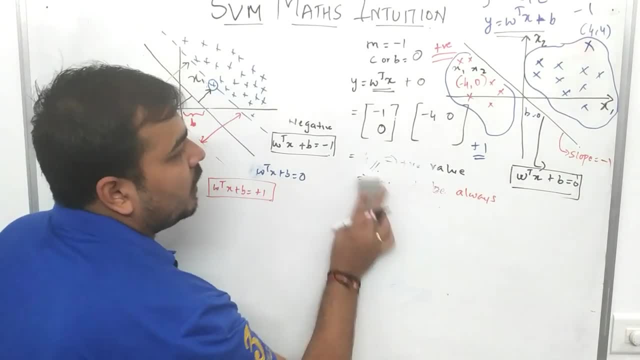 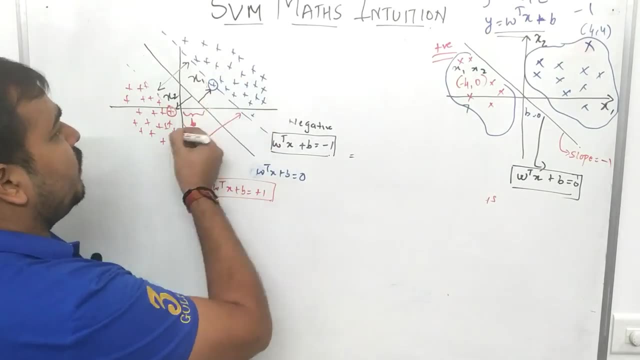 How do I compute it? just understand the way I'm just going to rub this, but I hope you have understood what I am trying to explain. Okay, let's go ahead Now. in order to compute this for this particular point, can I write the equation something like this: 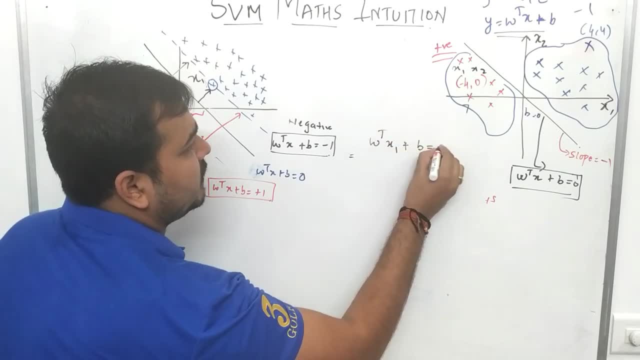 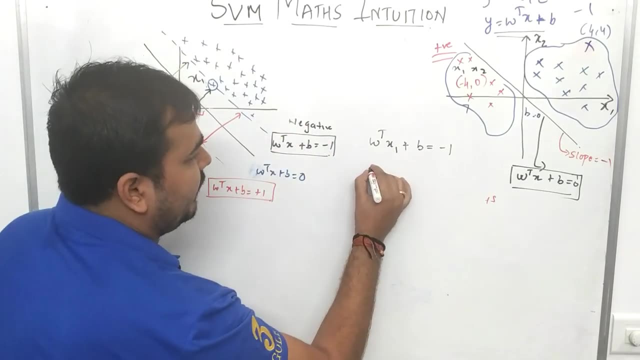 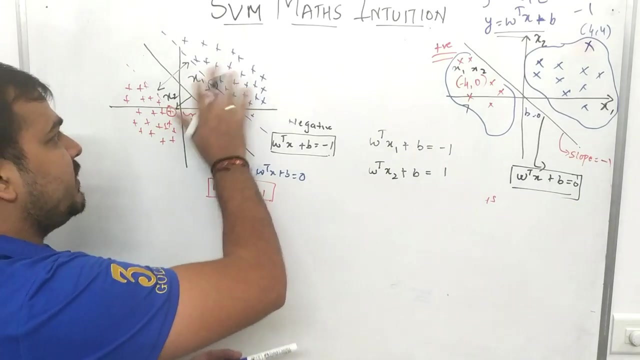 W transpose X, 1 plus B is equal to minus 1, because this is a minus 1, right, Okay, and for this particular point, I can write: W transpose X, 2 plus B is equal to 1, pretty much simple. I want to compute the distance between them, what I'm to compute, what is the difference between? 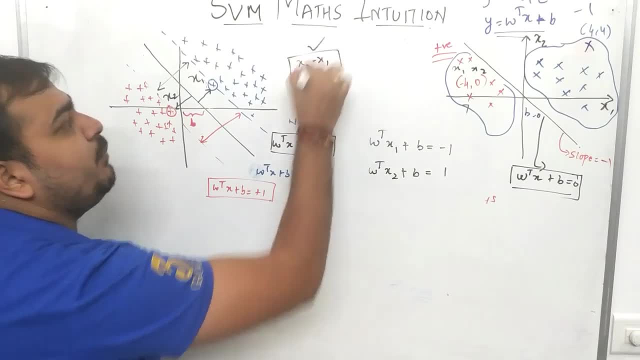 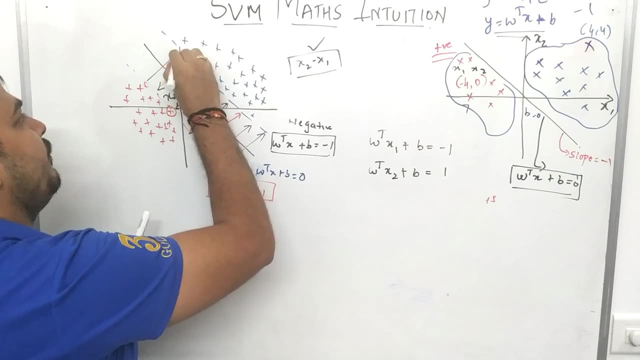 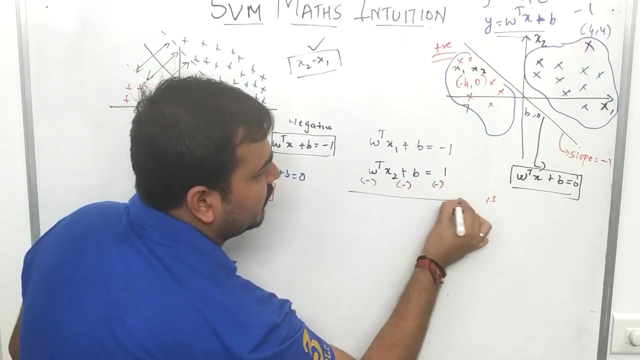 X 2 and X 1. Right, This is what I want to compute. that will actually give me the distance. Remember: all this distance are same. if I consider all this particular distance, they are same. Right now, when I am computing this, Let me just write it as minus 1, minus 1 over here, because I need to find X 2 minus X 1. 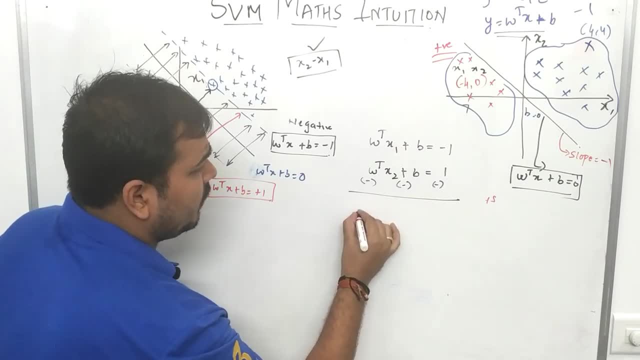 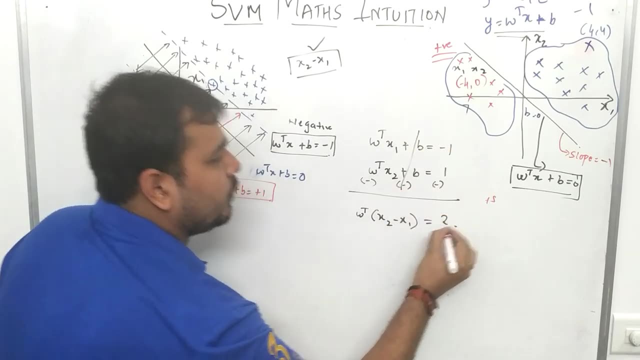 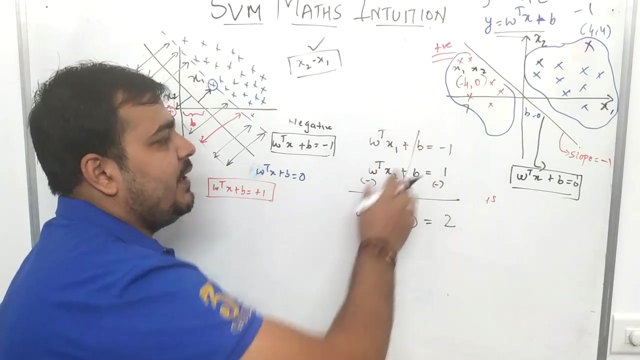 So over here you can see that I will write it as the W of T X 2 minus X 1. this will get deducted and this value will be 2. pretty much simple what I've done. I've just- I Hope you have done this in linear algebra, right, normal? I've just taken it. 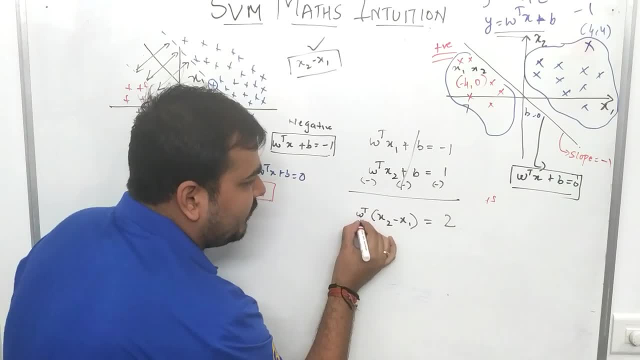 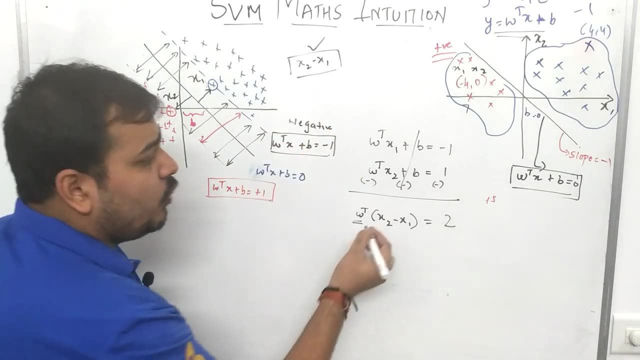 I want to find X 2 minus X 1. now, now understand. I just have this W of T. I need to remove this. W of T is nothing but this transpose of this particular slope values, And if I want to remove this, I can actually remove it with the help of norm of W of T. 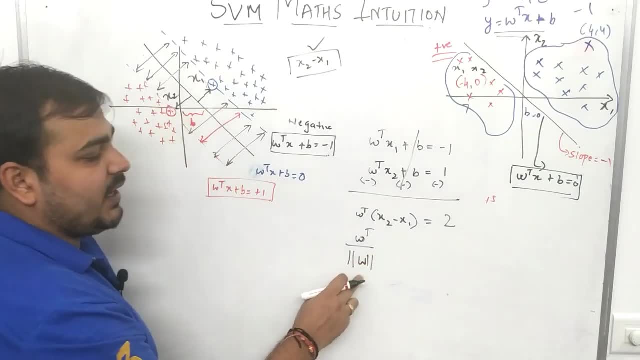 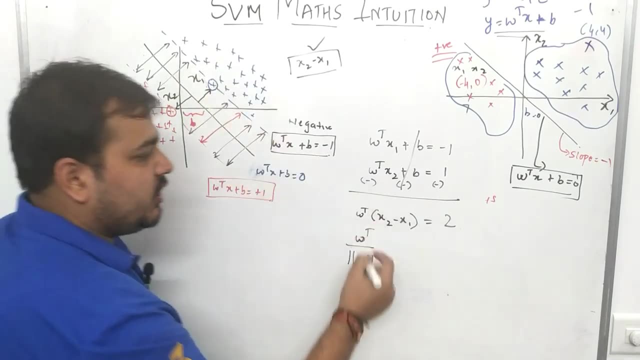 Norm of W. norm of W basically means we are given by this particular notation. I cannot just write directly: remove W of T, because there is some direction involved. Okay, there is some direction involved. So for this, what I'm going to do, I'm just going to write like this: I'm going to divide by 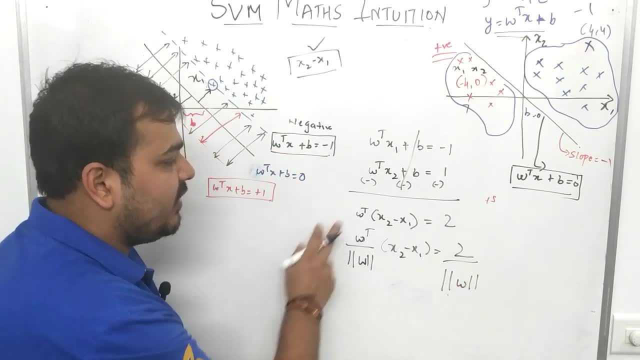 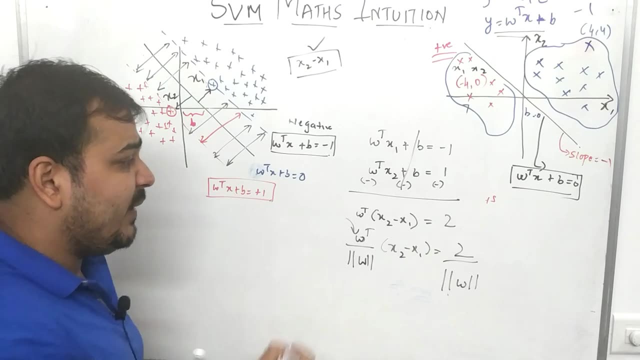 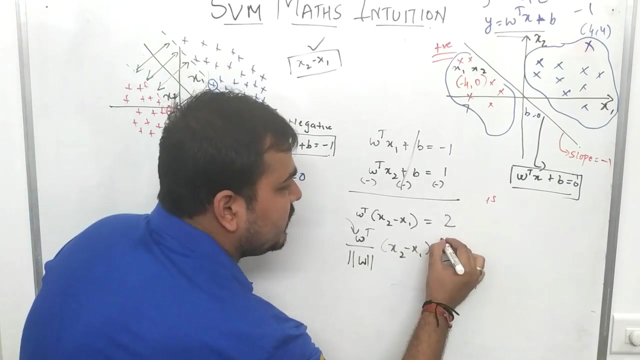 Norm of W, Both the side I am dividing by norm of W- that, basically, as soon as I divide this, this, this whole magnitude of W Will just go off. this whole magnitude of W will go off, but there will be some direction: X 2 minus X 1, this direction that I am talking about. So, finally, what it says is that this is my equation, This is my 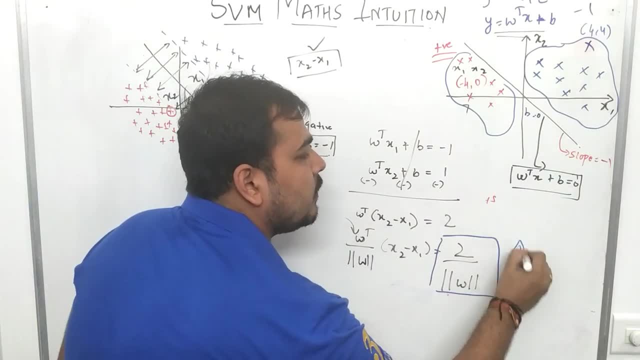 Optimization function and we need to maximize this. we need to maximize this. Very simple, again, understand. is we need to maximize this? Okay, so this is my equation, This is my optimization function and we need to maximize this. very simple, I can understand. is we need to maximize this? okay? 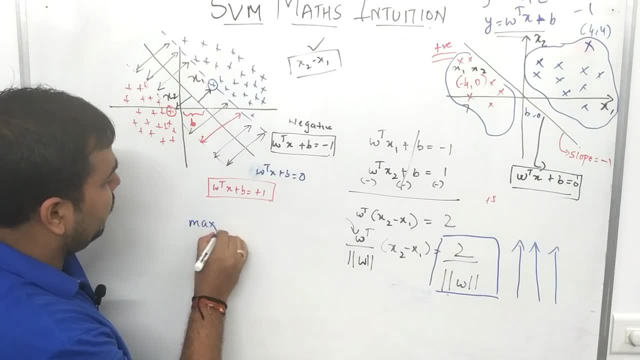 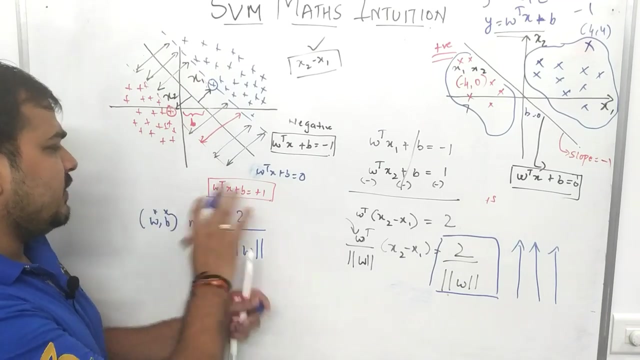 So let me just write it down again: I need to find out max. I mean, first of all, I need to update W, comma B, such that You know I have to maximize this particular value. Okay, pretty much simple. This is. this is what is my optimization function. 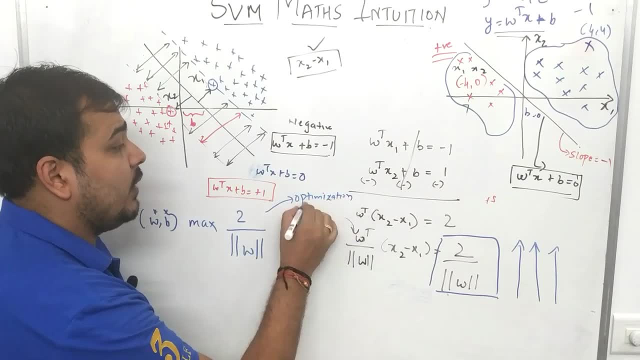 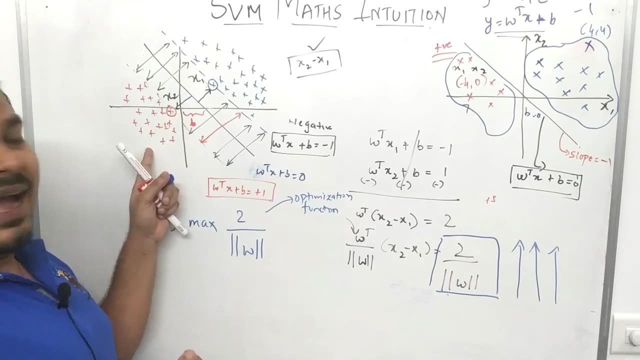 optimization function. But still, there is one more thing to consider over here. This is also. there is also one more thing to consider. I told you that anyhow I get the positive or the negative value, it will always be going to considered as minus 1 or plus 1, right? so here I will be writing such that: ok, let me. 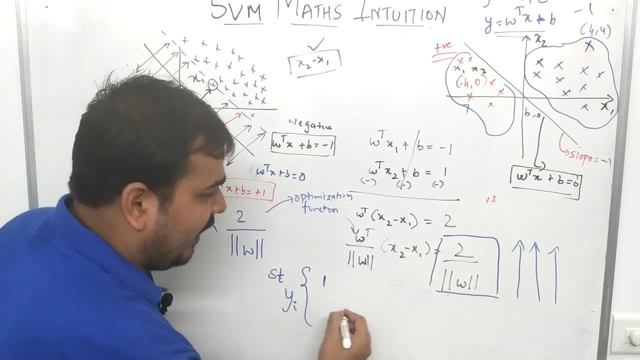 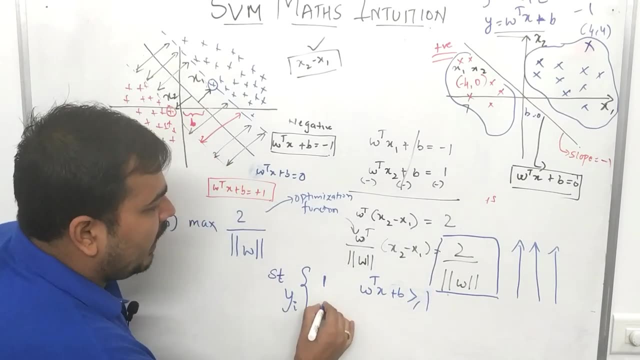 write my y of i will be 1 will be 1 where my wt of x plus b is greater than or equal to 1. ok, and this will be minus 1 where wt of x plus b is less than or equal to 1. sorry, 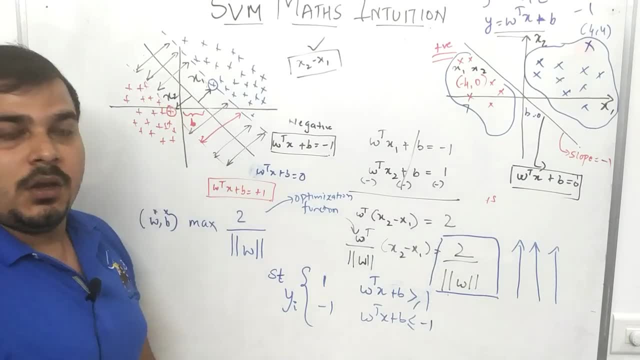 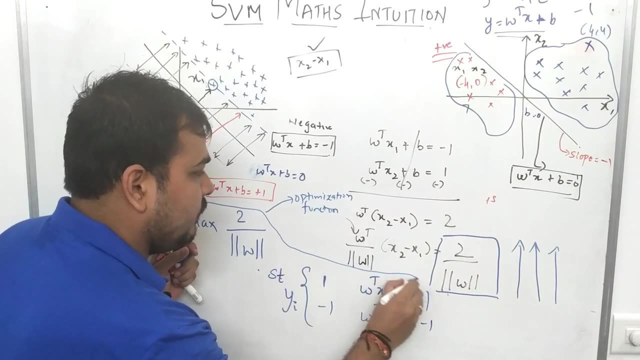 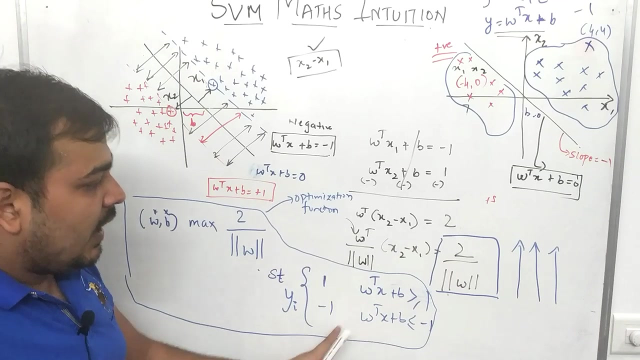 less than or equal to minus 1. ok, so this is my condition: I have to maximize this particular value. I have to maximize this particular value. ok, I am just going to draw it over here. I have to maximize this particular value, but my condition such that I always have to make. 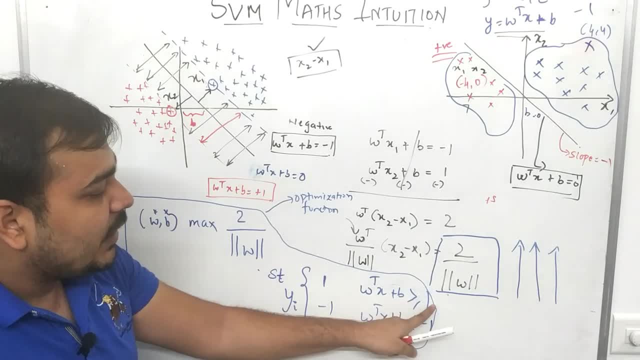 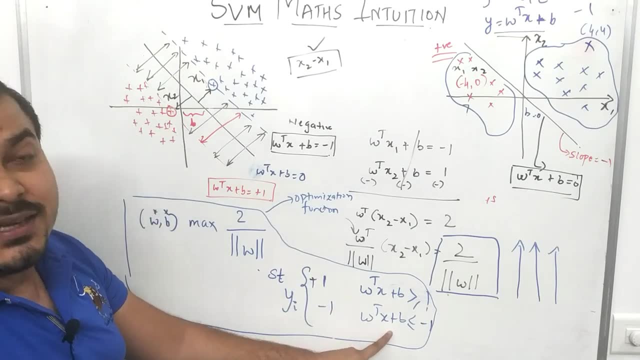 sure that whenever wt of x plus b is greater than or equal to 1, I have to consider my y i value as plus 1. ok, this is my plus 1. and wherever my wt of x plus b is greater than or equal to minus 1, I have to always consider this as minus 1, because that is what it says. 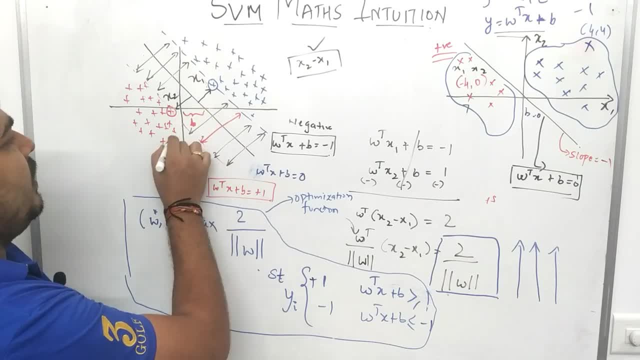 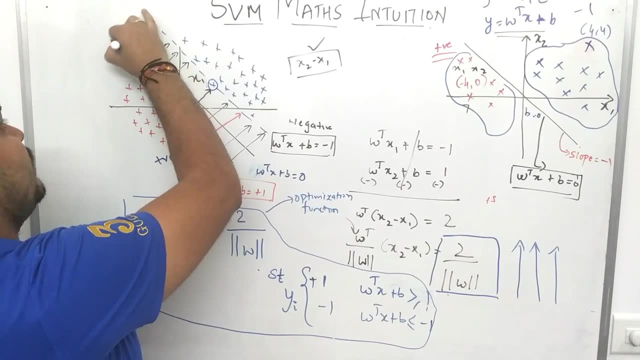 suppose I want to compute this particular distance from this particular point right here. I will definitely get a higher positive value, right? higher positive value with respect to support vectors: I will definitely get it as 1. with respect to this support vector, I am going to get it as minus 1. but what about these all points? I am going to get a higher. 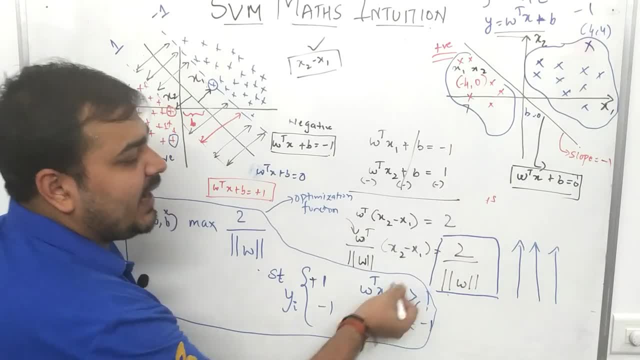 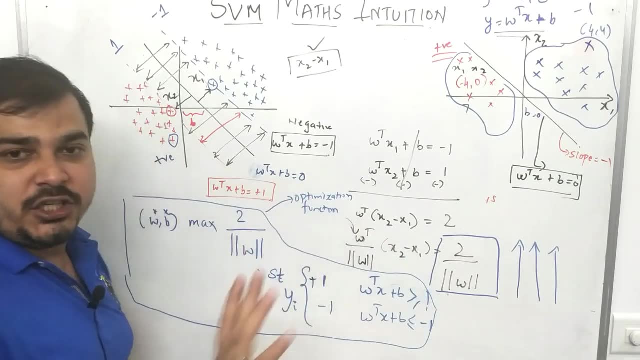 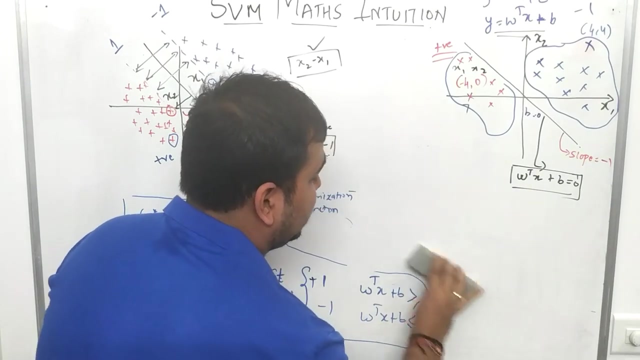 positive value. ok, with respect to this particular equation, whenever I get a higher value, I am just going to consider it as 1, ok, And that needs to be added. so this is my condition of my optimization, right? I am just going to rub this again. I hope you are understanding it, guys. if you are not, please just go behind. 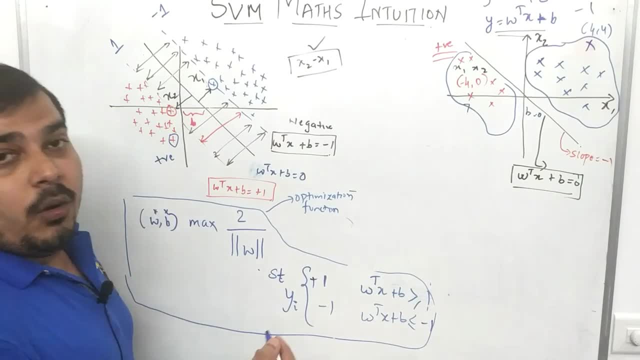 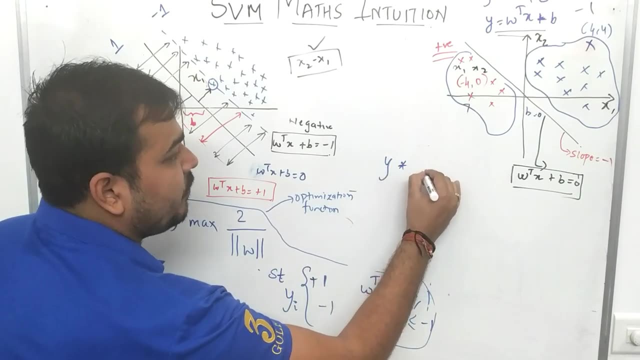 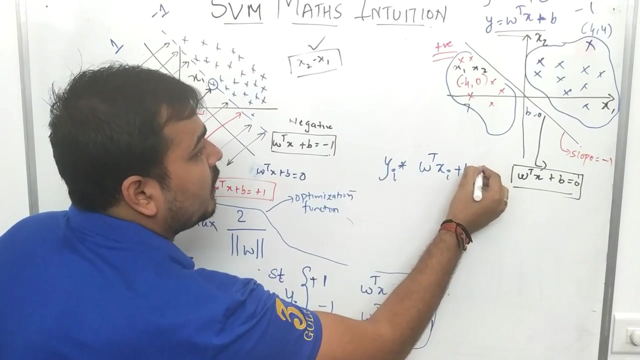 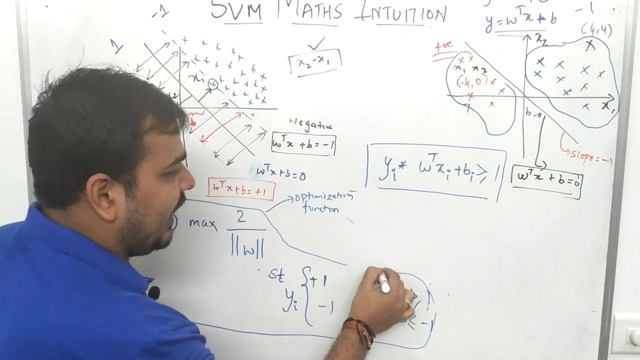 this and just have a look. ok, now I can consider this whole thing that I am considering such that right. I can also write: w multiplied by wt of x of i plus b of i is greater than or equal to 1. instead of writing like this, I can also represent it writing like this: why? 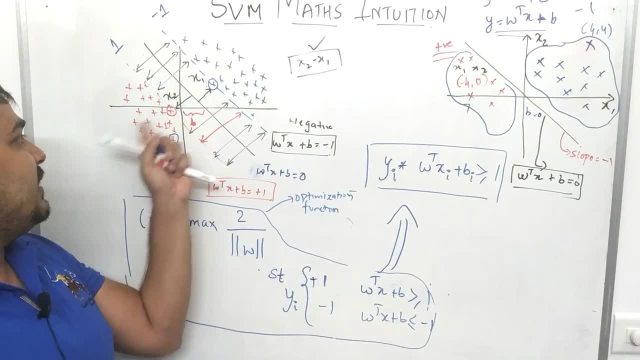 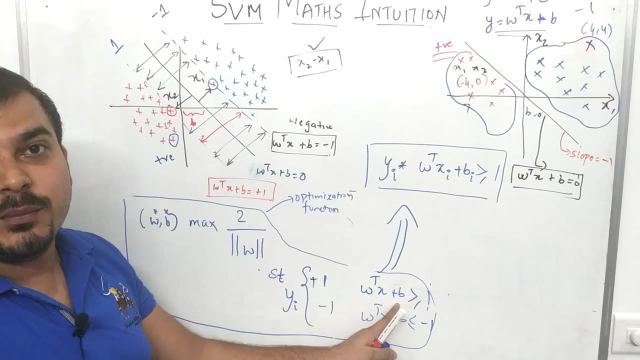 understand w of i. whenever I am computing, in this case it will be positive, right, and whenever I compute this right, if I compute this, this is also going to become positive. so anything multiplied positive, multiplied positive will always be greater than equal to 1, right. in the second case, suppose if my w of i is minus 1, minus 1, basically. suppose. 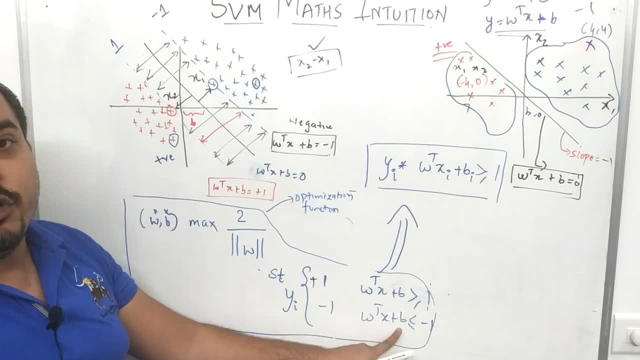 I am representing this point. Ok, and if I try to compute wt of x plus b of this from this particular distance or with respect to the y value, this is also going to become negative value. so negative value multiplied by negative value will always be greater than or equal to 1. now my main aim. 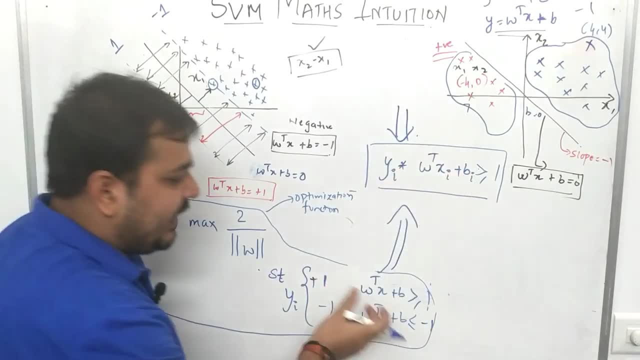 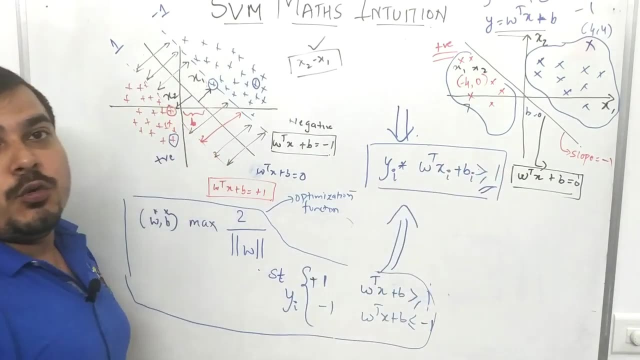 is that whenever I come to this particular equation and whenever I take this y value and this particular value, if I try to multiply, this should be greater than or equal to 1. if it is not greater than or equal to 1, that basically means it is a misclassification. 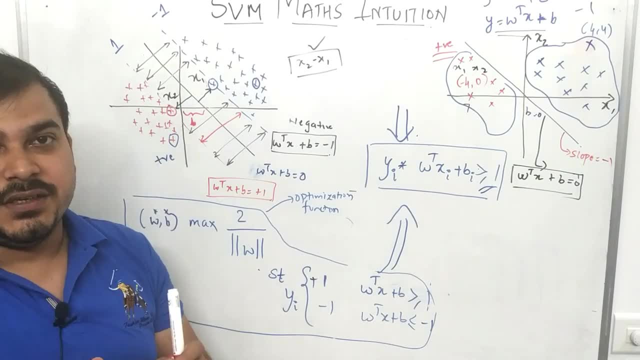 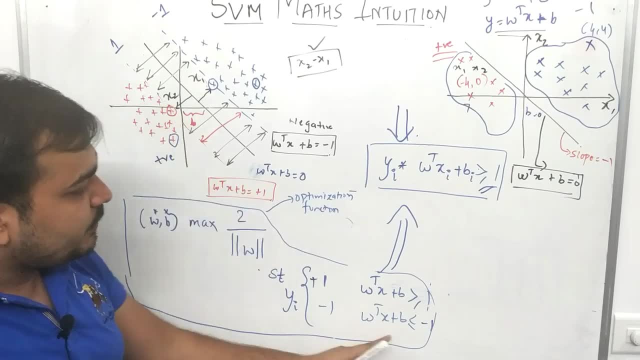 negative point is over here and when I actually compute this particular value it is going to become positive. so negative into positive will actually give me a negative which will not satisfy this condition. my condition is that whenever I multiply this value with this value and this value with this value should always be greater than or equal to 1 in this. 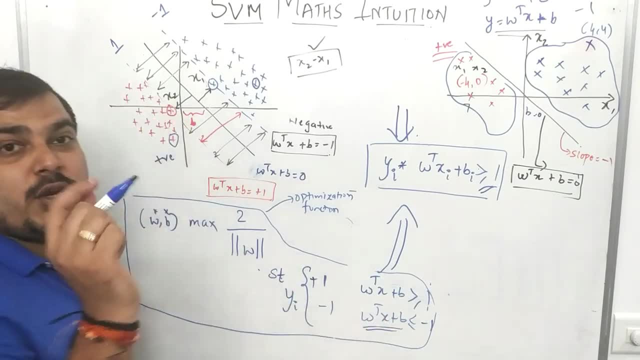 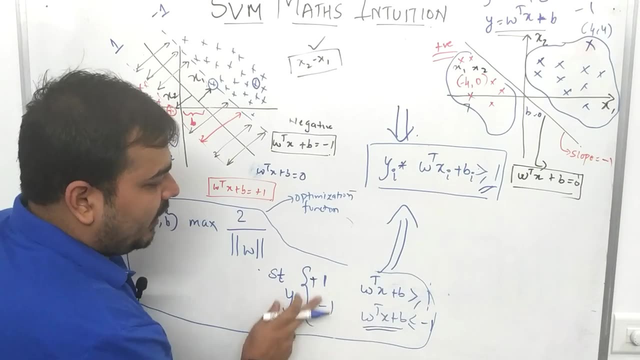 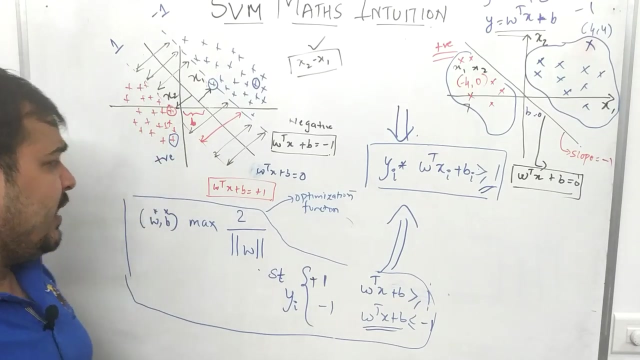 particular case, when I compute this for a negative value, this is going to become a negative value itself. I have shown you in this particular example, right in this particular example. so this multiplied by this will always be a greater or equal to 1.. Now, one more thing that is pretty much important to understand. this is my whole optimization. 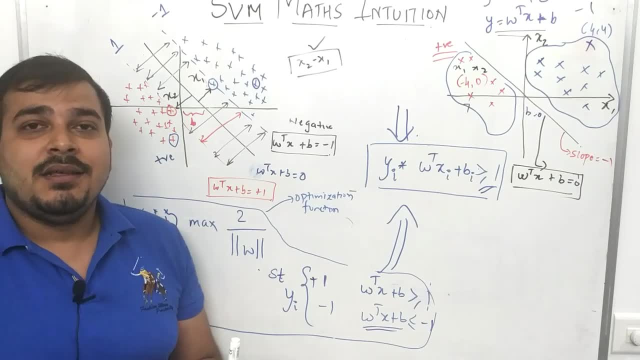 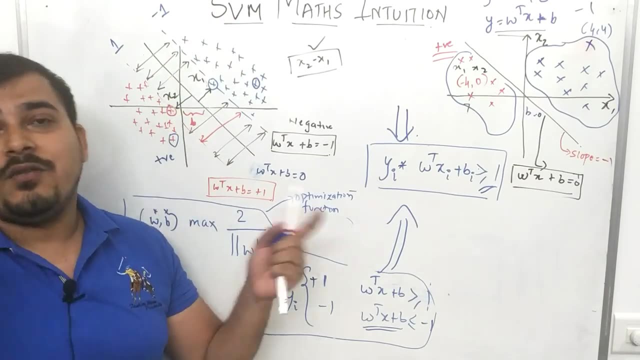 function right now. one scenario will be that always remember, in the real world scenario, I don't have this kind of points. we will not usually have this kind of points. there will be a lot of over lappings. there will be a lot of over lappings. 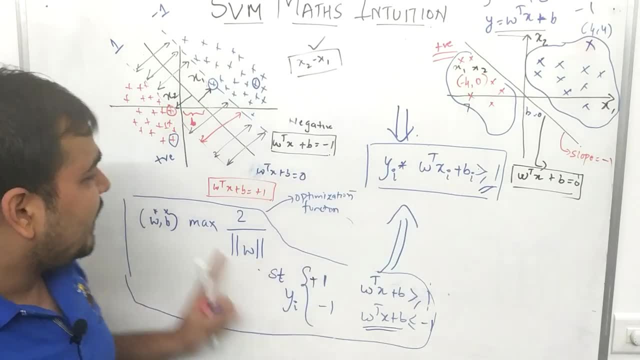 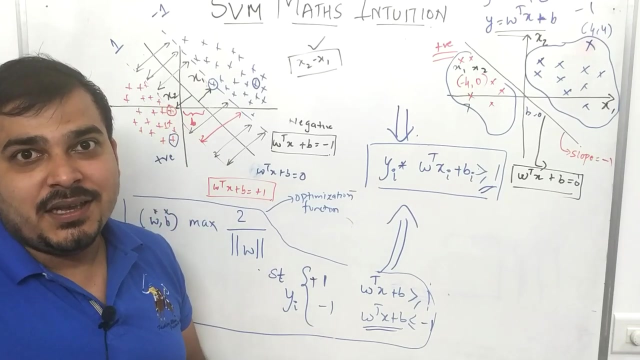 You know, If we try to get a situation in this particular way, that basically means we are trying to over fit the data. so in that specific way, we should just not over fit the data. instead we should try to find out a solution, or you can also say a hyper parametric tuning techniques. 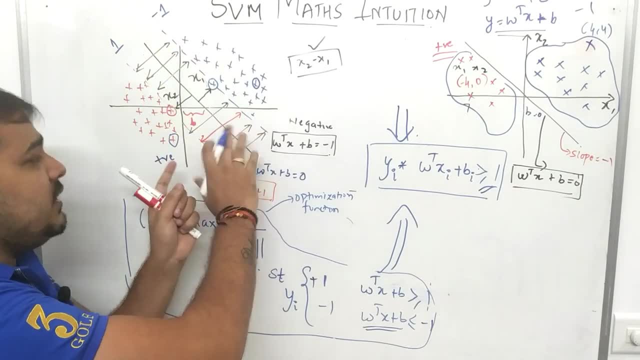 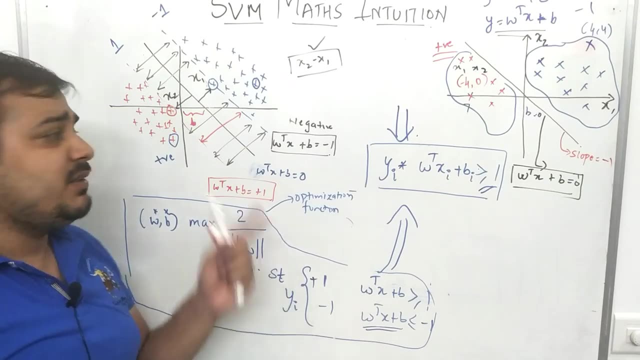 you know, because in real world scenario I will not be finding this proper way of, you know, a linear distribution. that basically means just by creating a straight line. I cannot divide those points. there will be a lot of over lappings, a lot of over lappings. 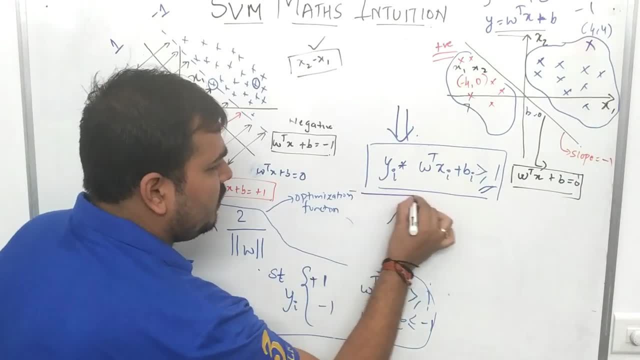 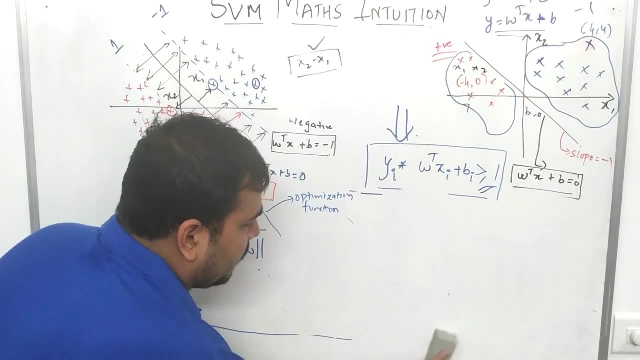 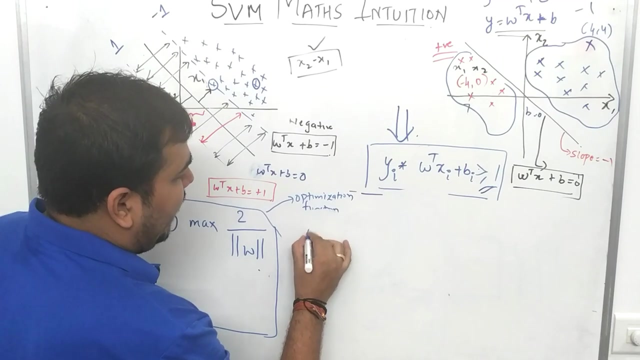 So what we do? is that the final thing about this particular equation? I'm just going to rub this, guys, because, again, I hope you have understood this, OK. OK, The final thing that I will write it as over here: Right, So I have to change W star and B star in such a way that not see, imagine way what I'm doing. 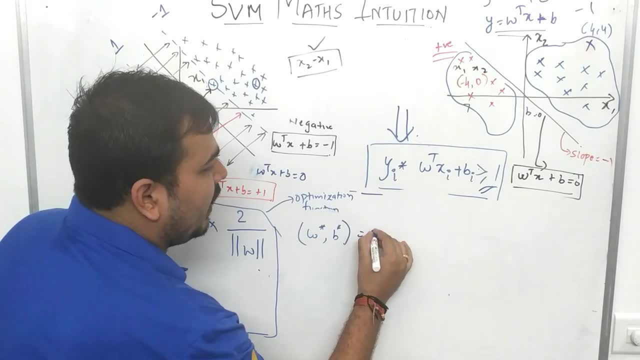 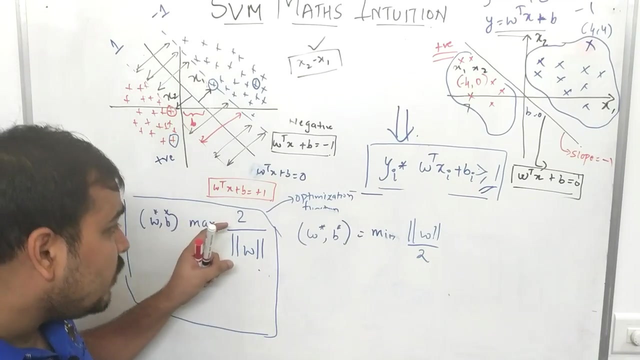 here max of two divided by norm of W. it is there. Now I will try to do mean of mean of norm of w divided by 2.. Now you are saying that. how did I reverse it? Understand for a function of property that whenever you are trying to do the reciprocal of the same 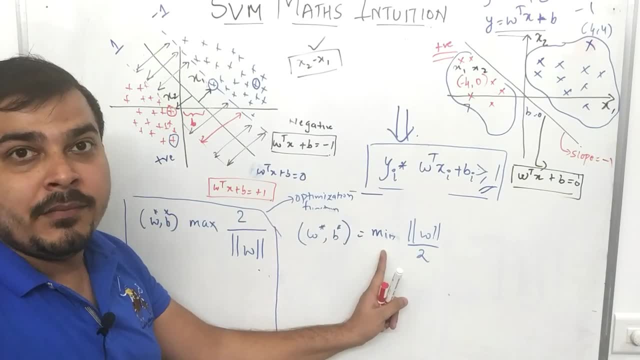 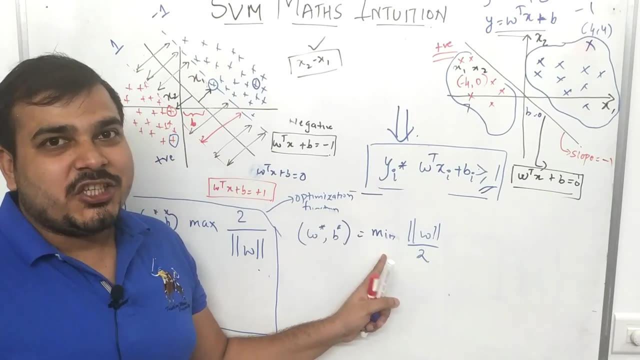 thing over here that instead of max it will become min. Now why I am taking min? because understand, guys, while you are creating a straight line also, and if you know about linear regression, there also we actually try to create a gradient descent In gradient descent also, we try to. 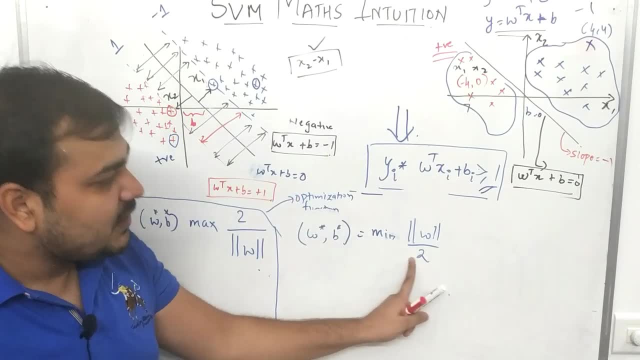 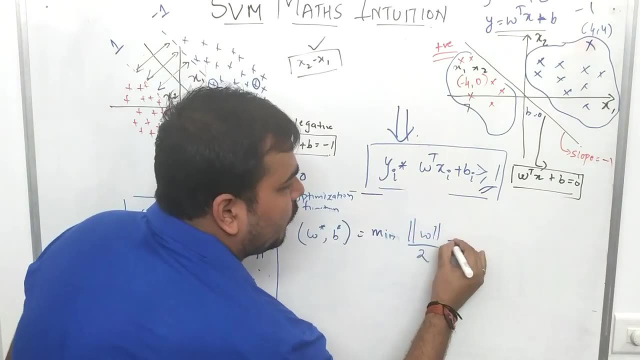 minimise this distance through derivatives. so that is the reason why I am taking this mean value, so this get be represented something like this. Now, apart from this, I am going to include two terminology just to optimise my model better. One is the C value. I will 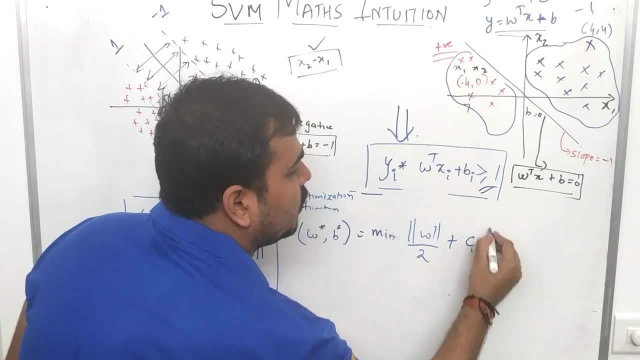 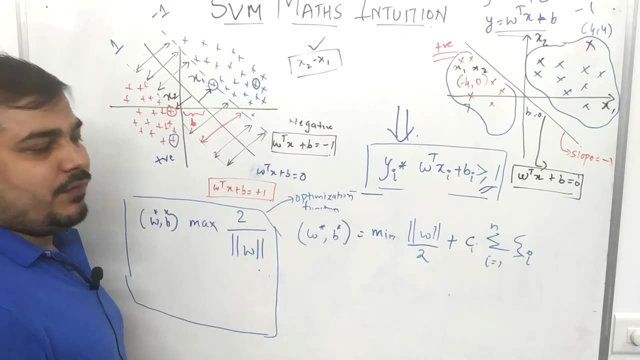 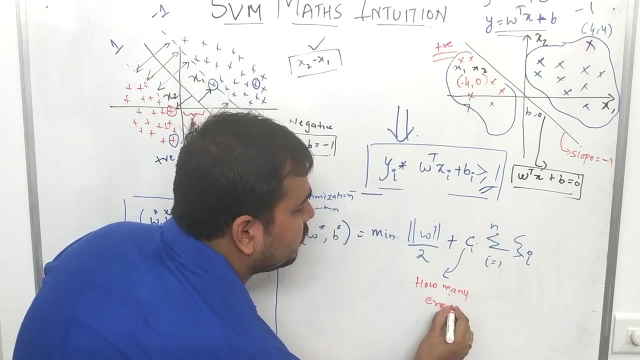 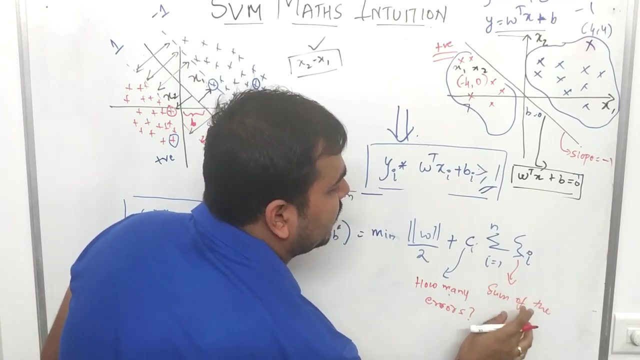 tell you what this C value is there and I is equal to 1 to n. I am just going to represent this as theta of. I Now understand what this two value basically means. C value basically says us how many errors my model can consider, How many errors, and this is the summation of or. I'll say that. 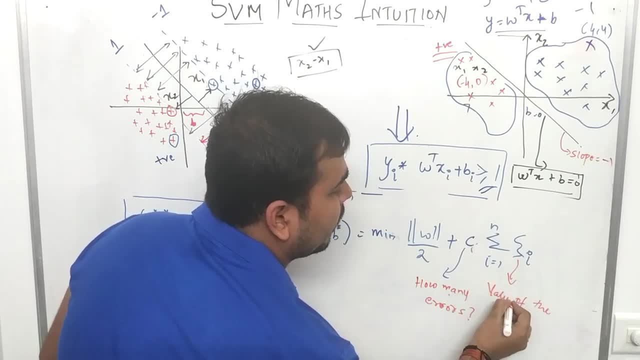 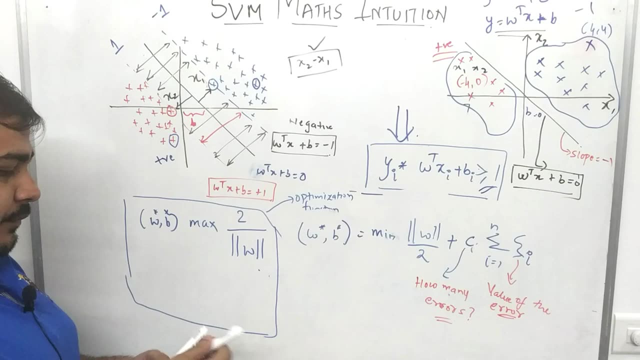 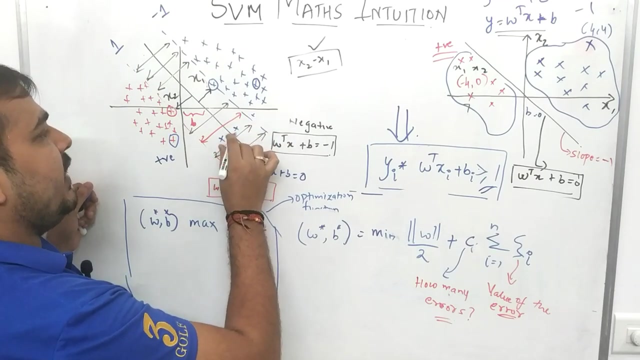 this. this is basically the value of the error, Value of the error. Now, this two terminology we need to understand. Understand over here, guys. suppose what is this? errors? Suppose this blue point is present below this line or over here, Right At this particular point. 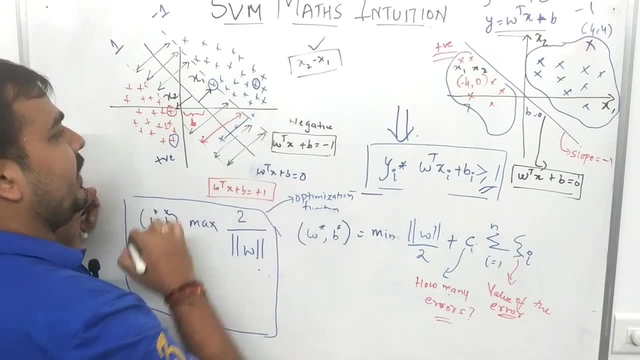 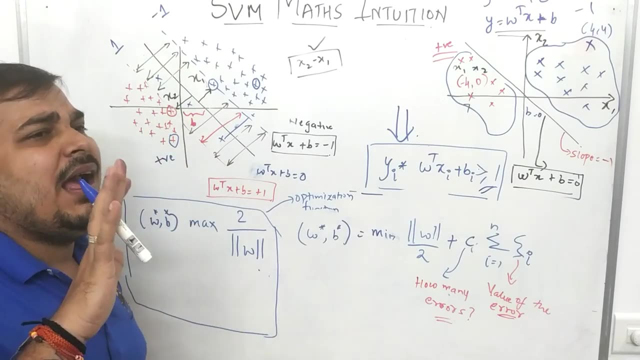 of time you can you know that this is misclassified, Right, This is misclassified. Suppose I may have two to three points. OK, And suppose my model, I'm considering that, OK, I can, I can say that OK, even though there is five errors, my model is not going to change this hyperparameter. 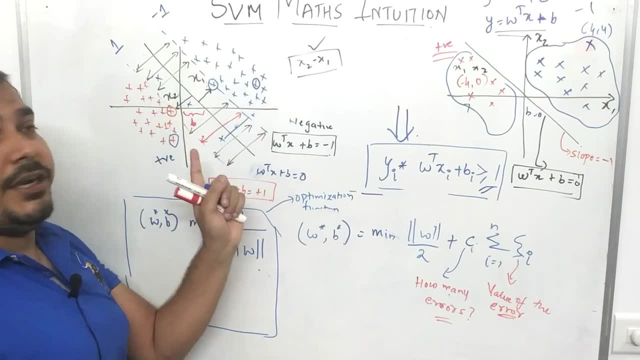 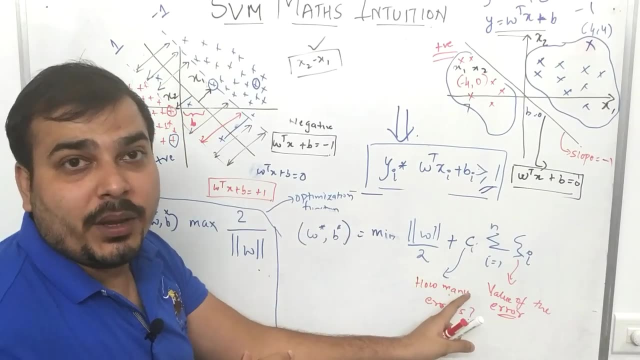 line, I mean the this line, this hyperplane. that divides the point. OK, I'm not going to change it. OK, It's OK. Fine, Two to three errors will be there, Right? So I'm considering in that particular way, So this C value, basically. 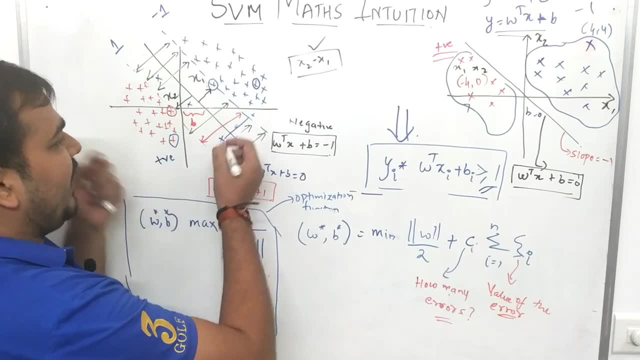 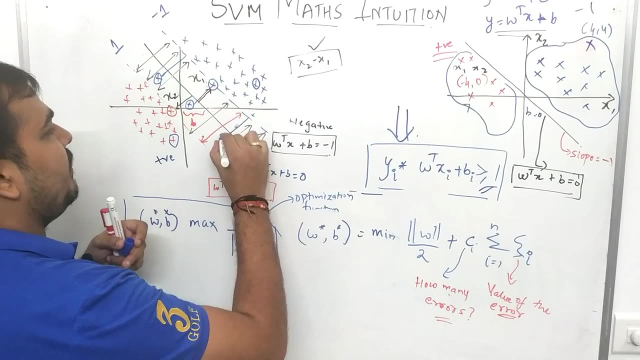 indicates that how many errors we can consider like this. Suppose I consider five errors, so three blue points I can consider: OK, This is basically an error Right. If I compute this particular distance, I'll be getting this as an error Right, And similarly I may have. 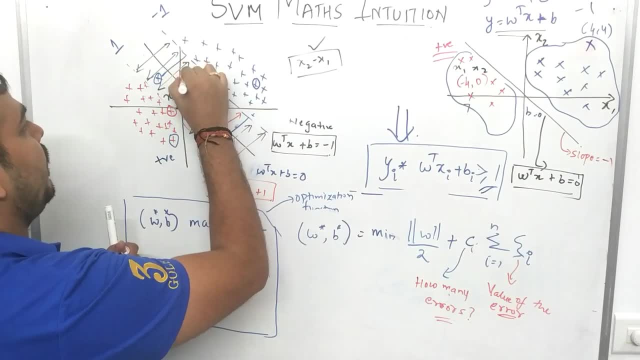 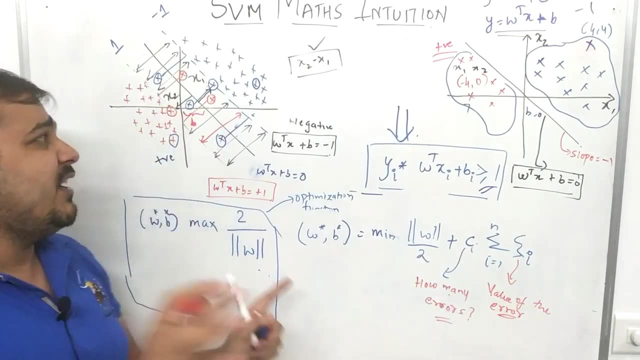 two red points over here. I may have two red points over here. This is also an error, Right? So I'm considering over here that my model can have five errors. even though I have five errors, I don't have to, you know, change my hyperplane. It's OK, It is having five errors, You know. 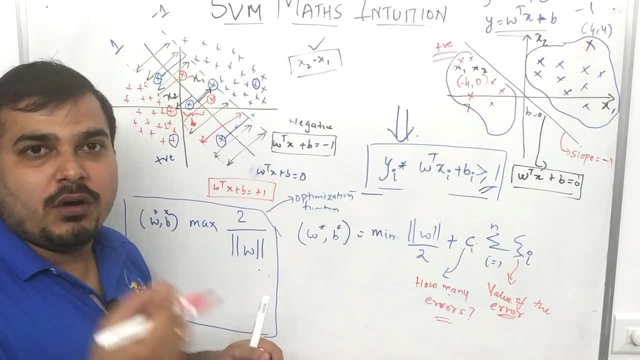 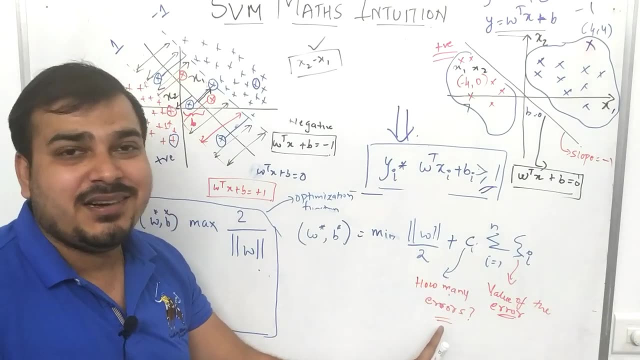 we're trying to fix the overfitting problem because if I try to do the overfit, even though I get one error, my hyperplane will be changing. That should not happen. I can consider some number of errors in my solution because I need to create a generalized model, Right? 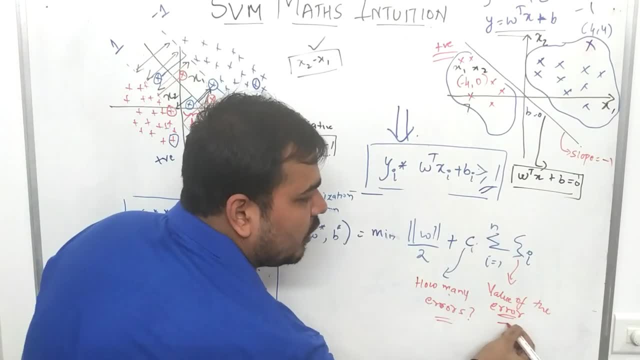 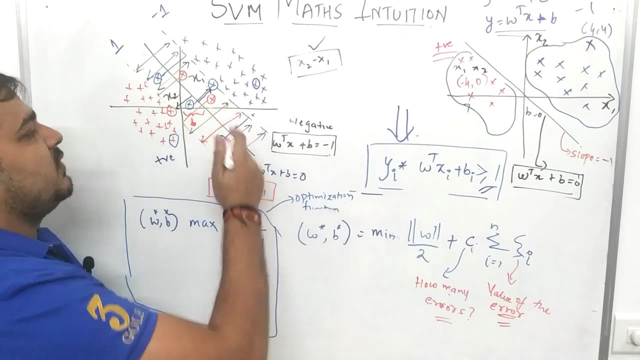 I need to create a generalized model. Now. the other thing is that what is the value of the error? The value of the error basically means that whatever distance I'm getting with respect to this error, I'm just going to do the summation Suppose for this error. I got five for this. 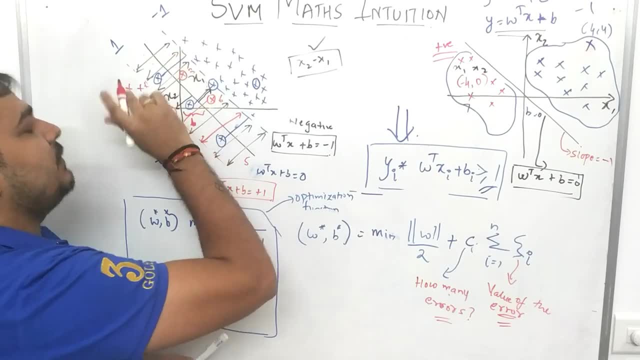 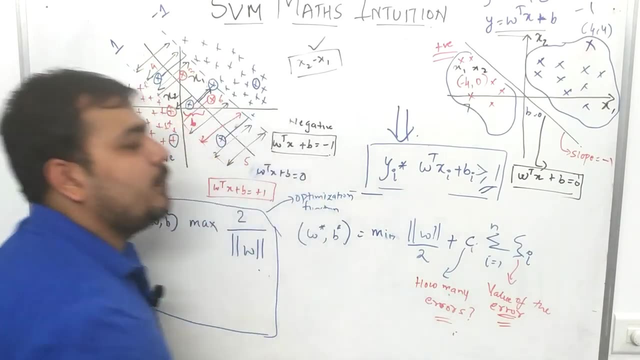 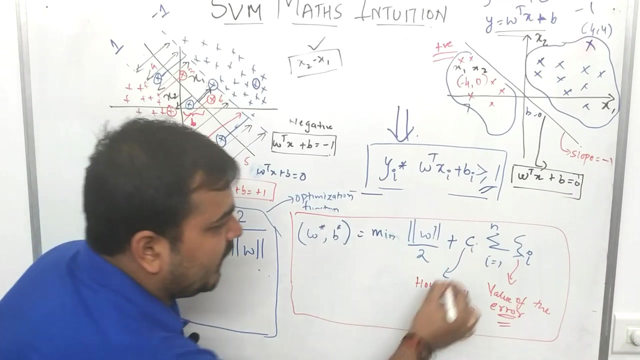 error I got six. for this error I got three. for this error I got, I mean, the value, the distance I got is as four. I'm going to add this: four plus three plus six plus five, multiplied by how many number of errors. So this whole is basically what is all about SVM, This particular 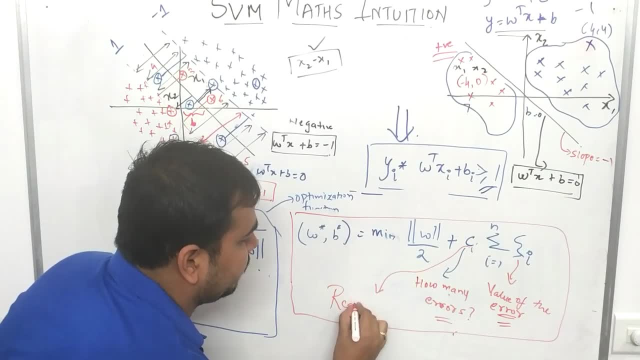 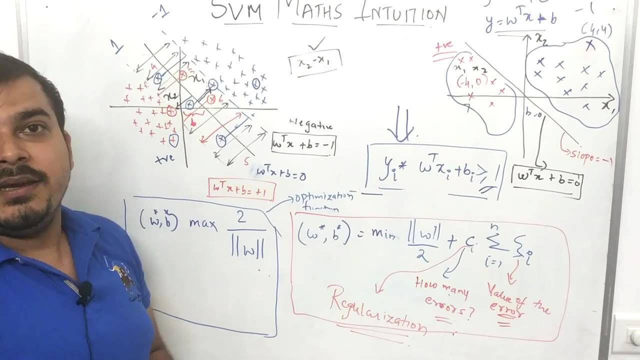 parameter is now called as regularization. OK, How do we get this value By hyperparameter tuning Regularization Right? So this is how SVM actually works. I know guys. there's a lot of maths included for me to learn. every time I learn SVM some new things. I understand about it And probably you have to see this. 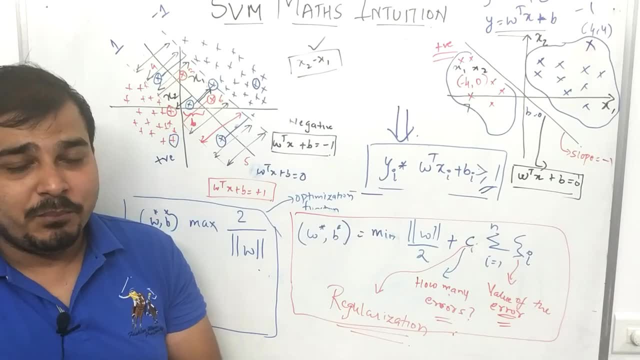 video again and again. I'm not demotivating you, But instead try to understand in such a way that you understand it, in such a way that you understand it, in such a way that you understand these things. Then only you'll be able to code much more efficiently. And 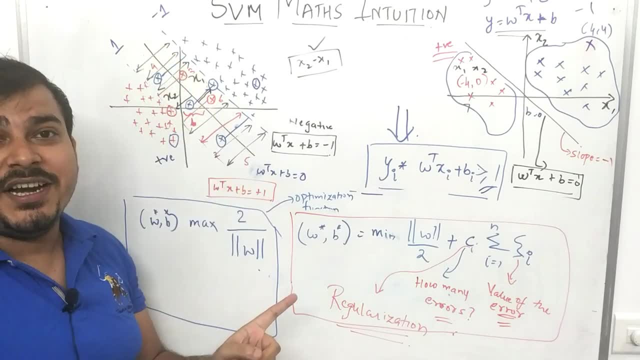 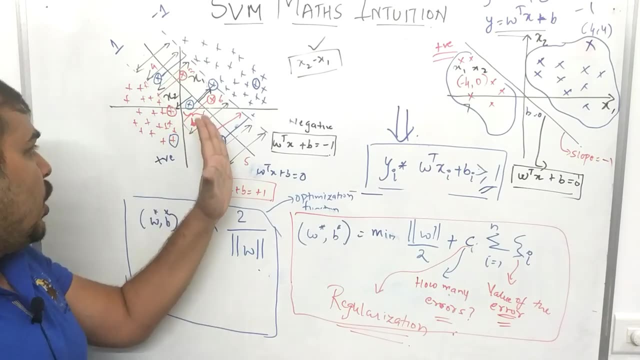 this kind of SVM. you know where we are just creating a straight line. This is called as linear SVM. You know hard, hard SVM We also call it. is that hard classifying SVM? That basically means we are strictly classifying all the points into two categories. Right, 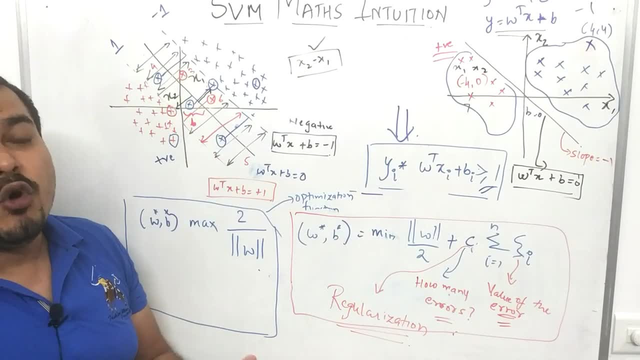 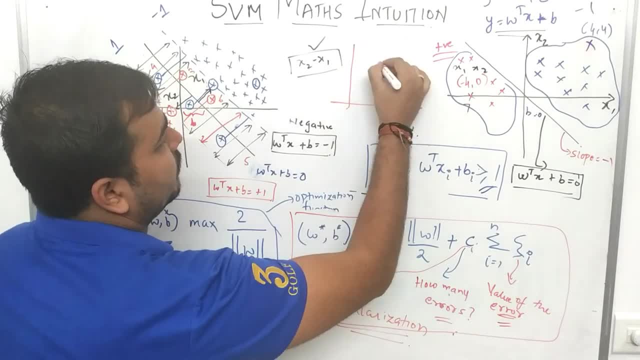 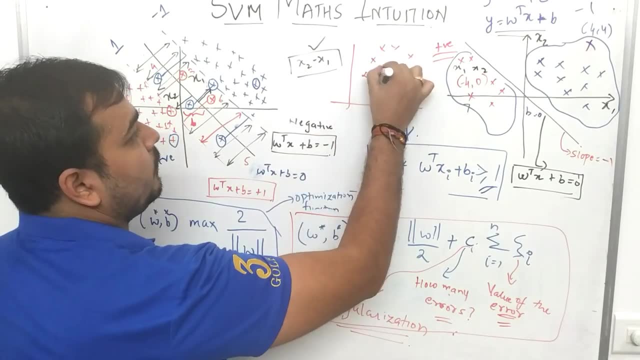 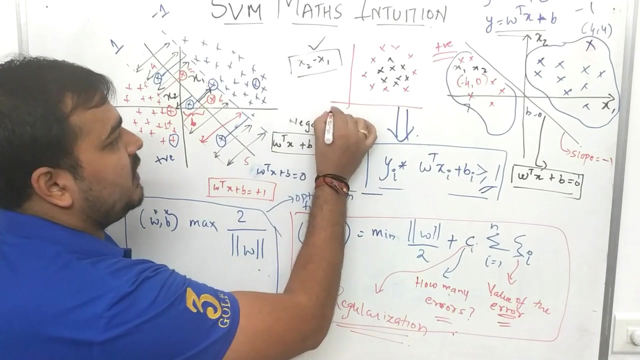 Right, Let me just give you one scenario which looks something like this: Suppose this is my points, Right, And you know I may have some other points In this scenario. I cannot divide these points and here I have to basically use the SVM kernel trick, The SVM kernel trick. 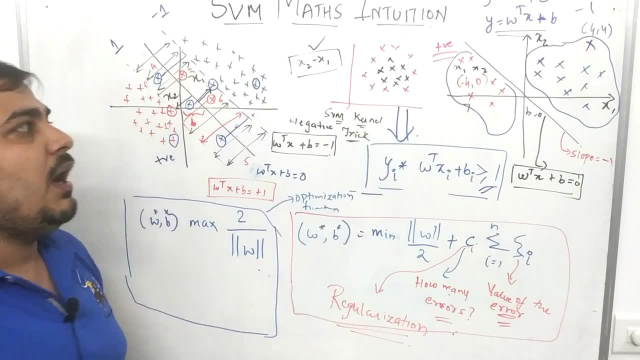 will be my next video. You know- and we'll try to see that- how we can solve this kind of problems where my data is not linearly separable. There is no non-linear separable data, Right, But this is how the maths is actually derived.